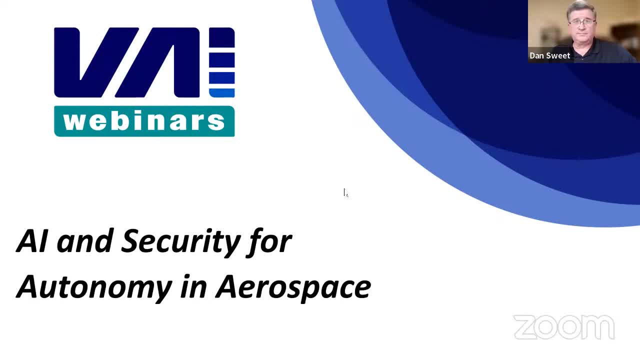 Hi, I'm Dan Sweet with Vertical Aviation International, and welcome to our weekly, or now monthly, webinar series. Today's topic is artificial intelligence and security for autonomy in aerospace. This is a topic that has been getting more and more attention lately. We actually did a webinar a couple of months ago on how artificial intelligence will be able to. 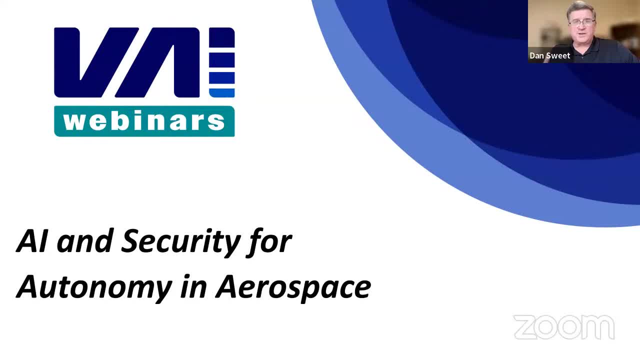 assist pilots in the cockpit. But just like everything else nowadays, where there is a very bright and positive outlook to artificial intelligence and use of it in our industry, sometimes there can be darker sides to it. And whether it's using AI to detect security, 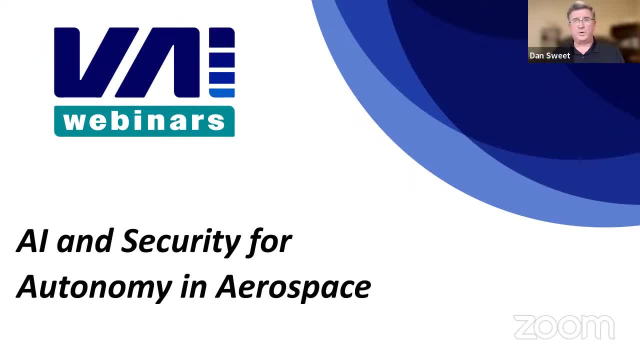 provide security for aerospace or the use of AI to attack aerospace. chances are somebody is going to be giving things a try, And so we thought it would be an interesting topic today to bring to your attention. So let's go ahead and get things. 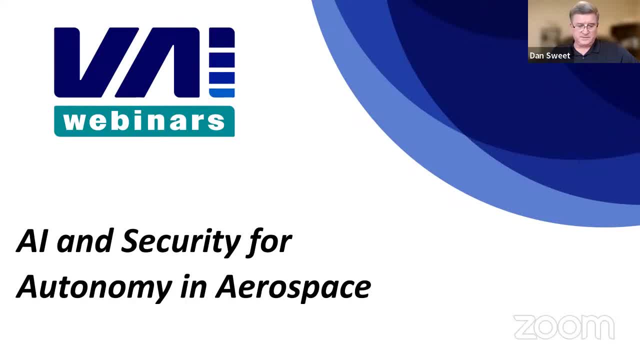 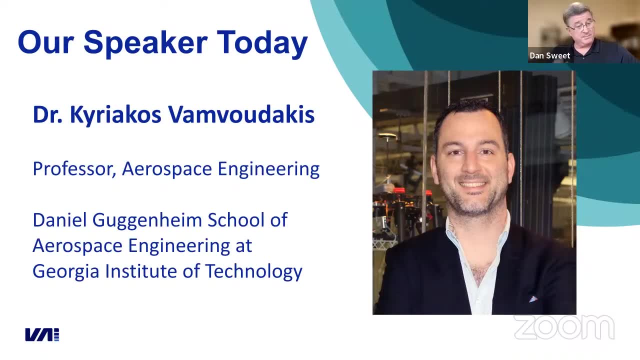 rolling See. here, there we go. Our speaker today is Dr Kiriakos Vamboudakis. I'm sure I just butchered that He is an endowed professor of aerospace engineering at the Daniel Guggenheim School of Aerospace Engineering at the Georgia Institute. 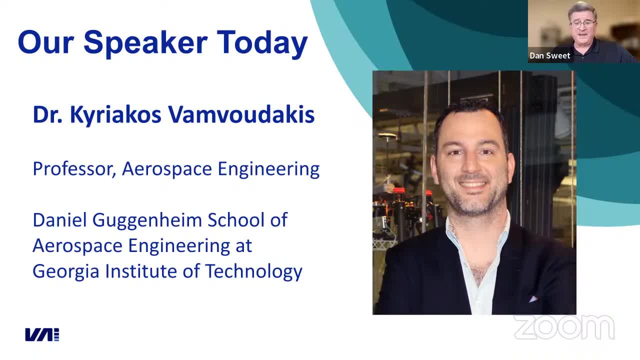 Technology, more commonly known as Georgia Tech. He received his bachelor's degree in electronics and computer engineering in Greece and his master's and PhD at the University of Texas in Arlington During the period of 2012 to 2016,. he was a project research scientist at the Center. 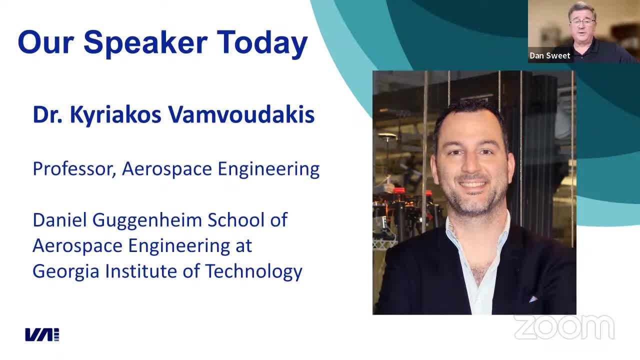 for Controlled Dynamical Systems and Computation at the University of California, Santa Barbara, And he was an assistant professor at the Kevin T Crofton Department of Aerospace and Ocean Engineering at Virginia Tech until 2018.. Vamboudakis is a highly accomplished in robotics and 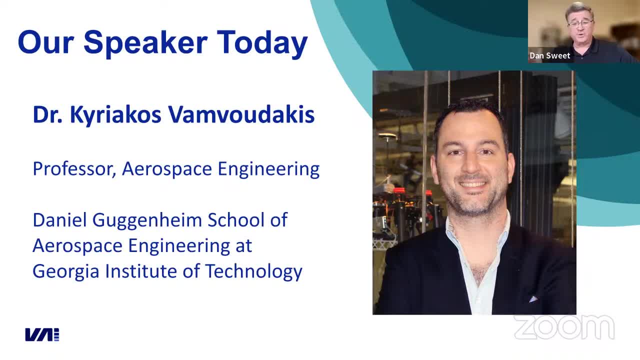 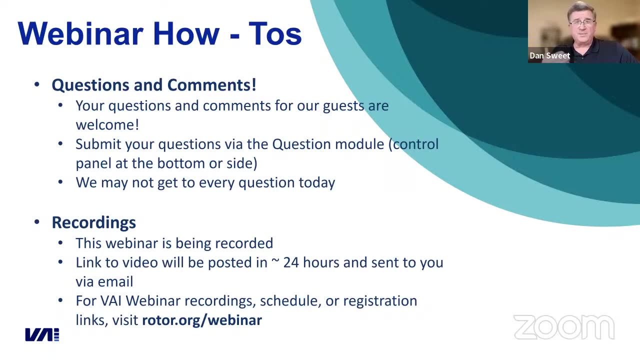 artificial intelligence research. In addition to his work here at Georgia Tech, he currently serves on NASA's secure and safe Assured Autonomy Project team. If this is your first time joining one of our webinars, we welcome you. We're glad to also have the people who have returned to. 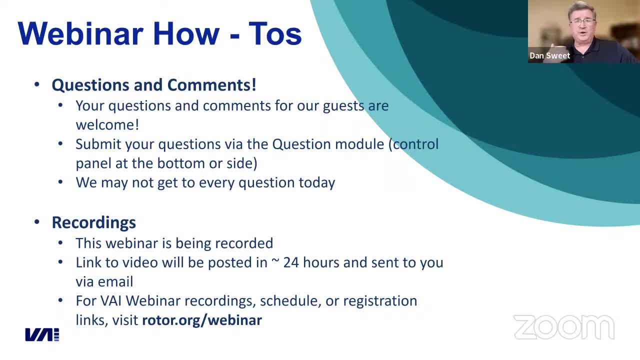 visit us, with us again. We encourage interaction on these webinars. This topic, I'm sure, can be fairly technical, And so if you have a clarifying question you want to ask, please do so. Please use the question module within Zoom, The chat feature. please go ahead and use it If you want to chat amongst yourselves. that's. 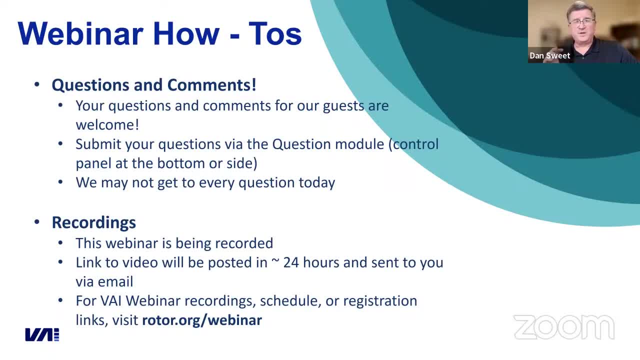 fine, Tell everybody where you're from, whatever you might want to do, But if you have a specific question on today's topic, please use the question module, either on the bottom of your computer screen or on the side of your phone screen, or wherever it might show up normally. 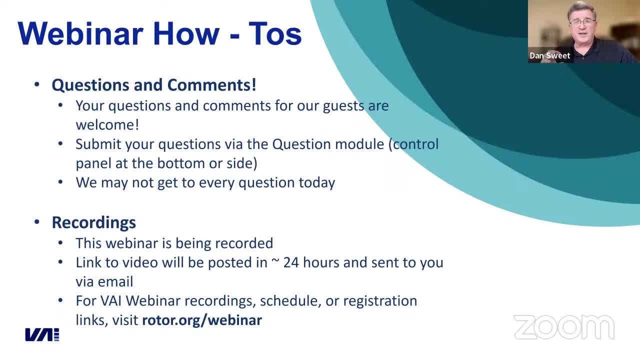 We will do our best to get through all the questions at the end of the webinar. We'll hold those until the end and then run through those. We'll see how we get to do on time. The webinar is being recorded today If you missed something, if you want to go back and review. 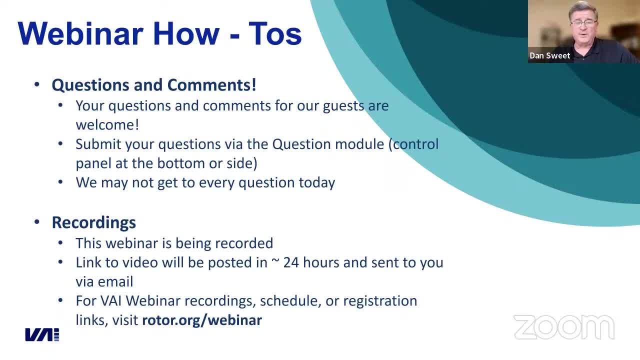 something, or if you want to share the video, which we strongly encourage. we know that not everybody can be online at the same time, especially midweek during the workdays on the East Coast, West Coast, around the world. We'll make that link available as soon as possible. If you have any questions, feel free to reach out to us. We're happy to help you. 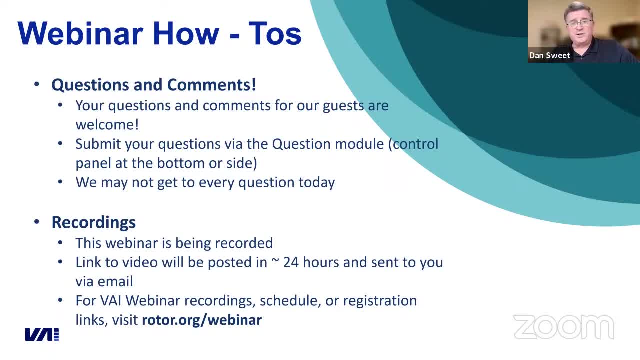 Thank you. We're very excited to hear from you. Thank you, Thank you. Thanks to all of you for coming. I appreciate it, So feel free to reach out to us And thank you to the team that has worked on this webinar. 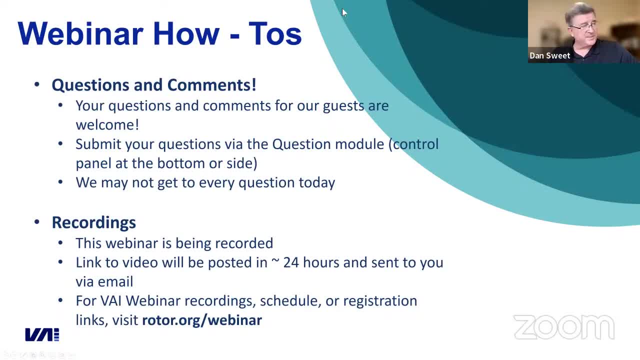 I will link this link as well as we possibly can, And that should either be tomorrow afternoon or possibly as late as Monday, depending on how long it takes to render and other technical issues. So let's go ahead and get started, Dr M. 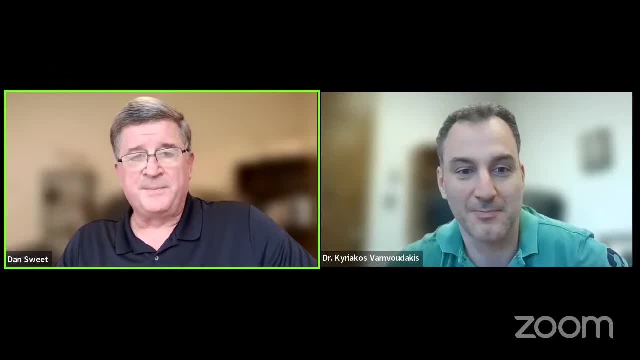 Mudeckis, welcome to our webinar. Thank you for taking the time out of your schedule to do this. Thank you very much, Don. It's a pleasure being here. Thank you for the invitation And thank you to everybody for being here. 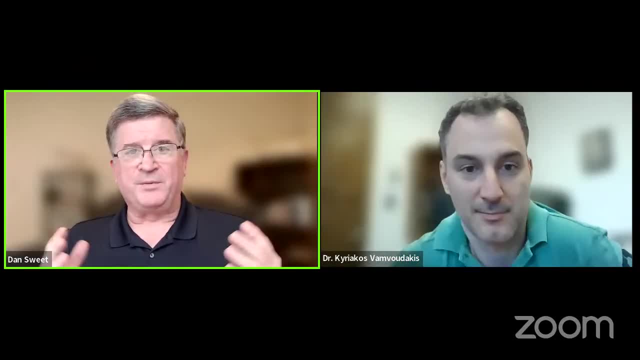 Well, you know, I think most people are most familiar with the importance of technical training and technical references with artificial intelligence right now through programs like ChatGPT, And we know that it was originally designed, I believe, ChatGPT to help coders. 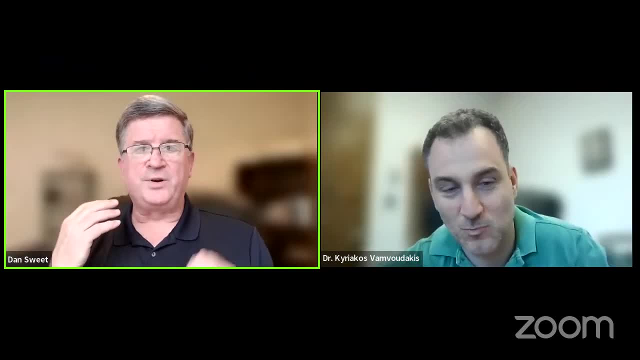 with some of their computer technology, And so there is so much work that artificial intelligence can do to benefit society. But again, there's obviously always a darker side, And it sounds like NASA and your team have been doing a lot of work to help try to make sure. 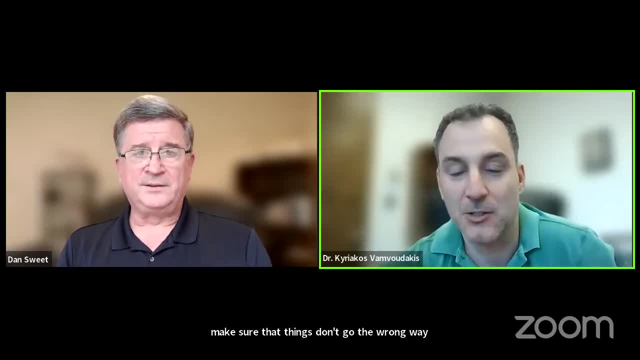 that things don't go the wrong way. Exactly, exactly, Yeah. So again, AI has been very popular nowadays, especially with all the computational power we have. So AI is nothing new, though You'll see in my presentation. So AI has been around for more than 30 years now. 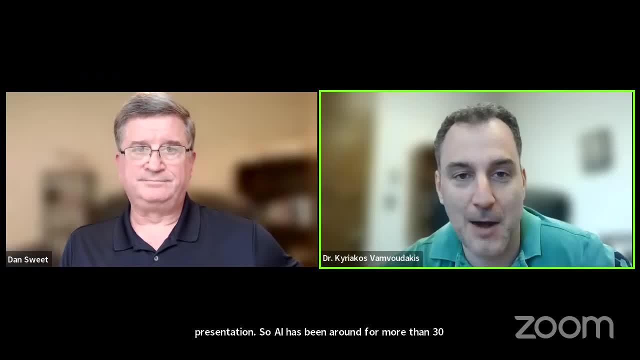 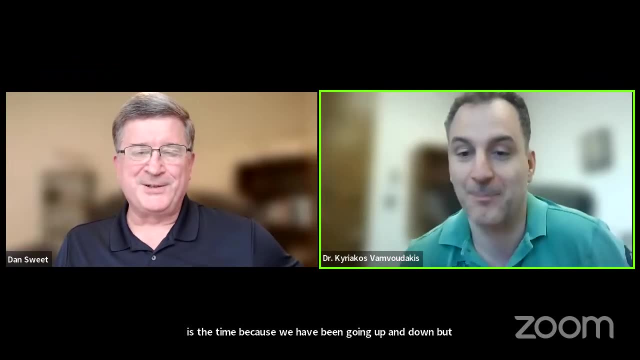 but it has been going up and down. But now is the time because we have all these components that we can solve very fast. So we have the computational power to do That. is true, My first time I ever played with a computer we had to load the program off cassette. 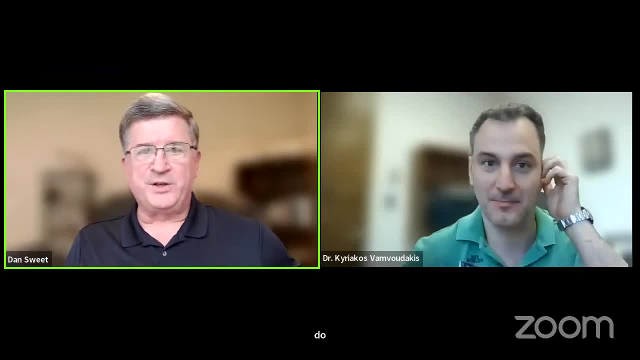 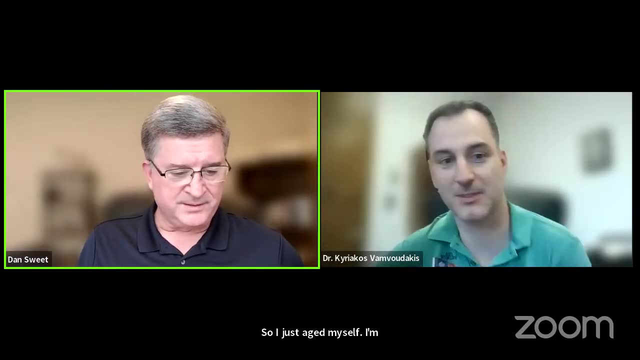 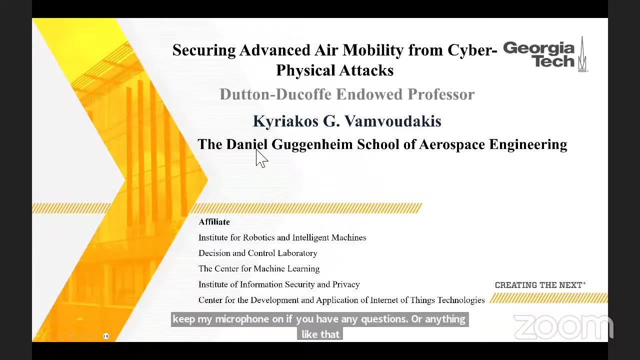 So I just aged myself dramatically. I'm going to go ahead and turn my screen off and let you go ahead and run through your presentation. I'll keep my microphone on. if you have any questions or anything like that, I think you can see my screen right. 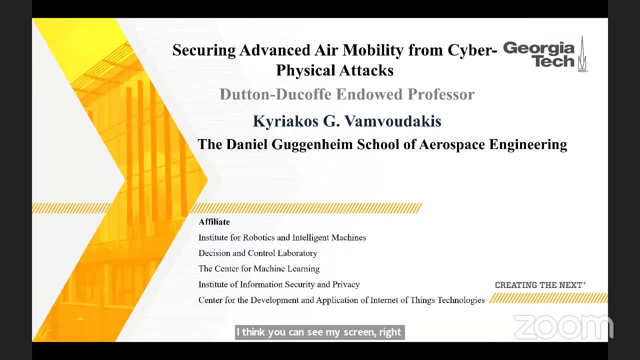 Your screen looks good. Yes, go ahead. Perfect, perfect Again. so thank you very much. So I will try to be non-technical. So that's probably one of the few times I give non-technical talks, but I'll try my best. 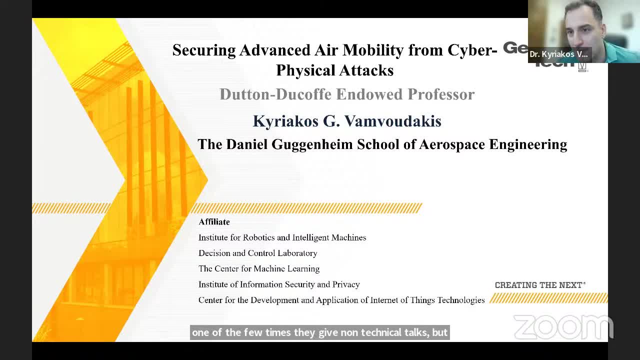 And again, I consider this as a discussion. So anytime you have something I will be happy to answer any questions you guys have. So, as Dan said, I'm a professor at the Daniel Guggenheim School of Prospects Engineering. I've been here for five years. 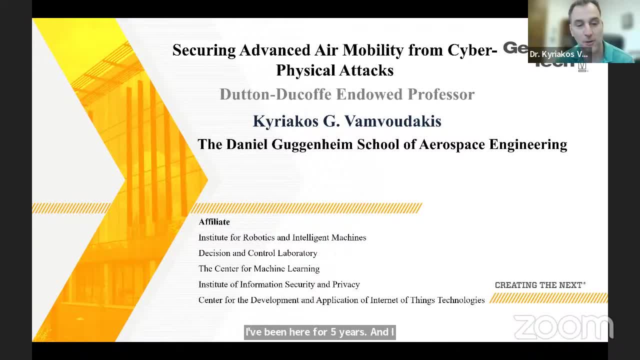 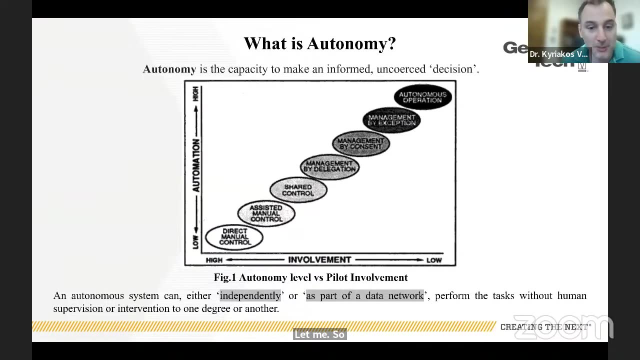 and I work on control theory, theory of autonomy and anything that has to do with security as well, for autonomy. So let me So, in this audience, I would like also to describe what is autonomy. okay, So autonomy- actually it's a Greek word. 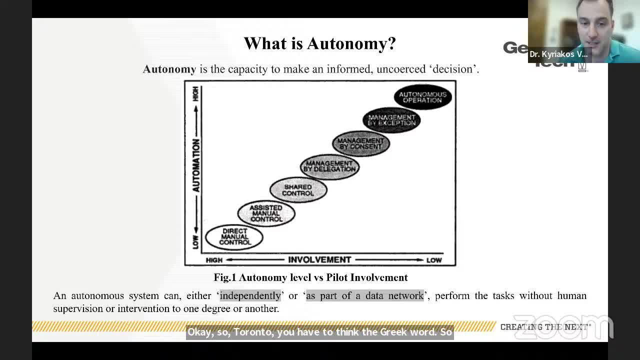 So it's the capacity to make an informed and encouraged decision. So here I found a very old figure. So where you can see that, the involvement- hopefully you can see my cursor- so the involvement from high to low, okay, So of course, when a person does very direct manual control. 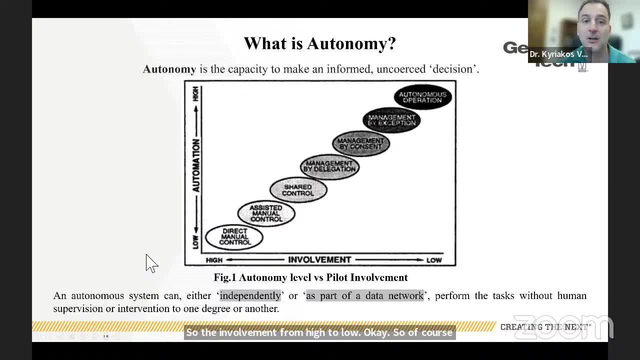 okay. so of course it has a high involvement And as I go towards high automation and high involvement, then I go to autonomy, okay. So you will see more about that. So, again, autonomy is anything that it is smart and doesn't involve any humans, okay. 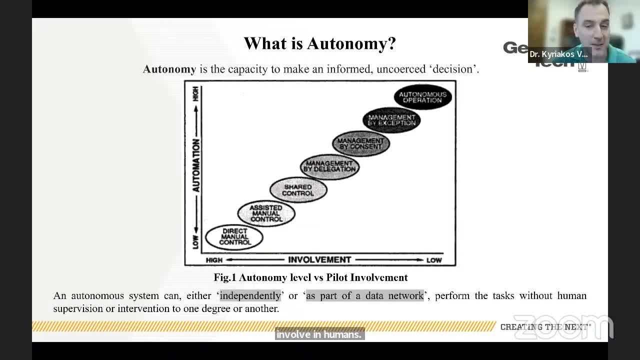 So somebody can tell me: okay, how about the Tesla? So again, that The human always has to touch the steering wheel, okay, And then it doesn't work properly in some streets, But we can talk more about that later. So, as Dan said, 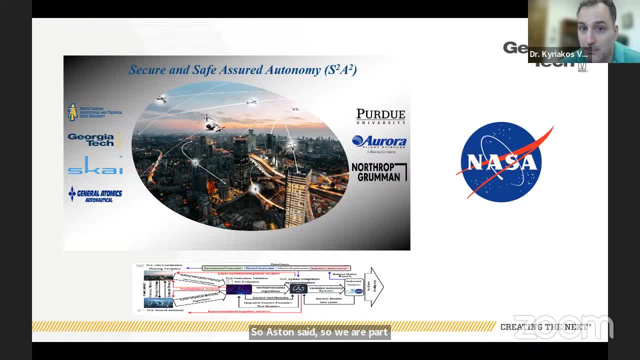 so we are part of a very accomplished team that we work on a very big project with NASA- I think it's about $8 million- And so it is led by North Carolina Agricultural and Technical State University. Georgia is part of the consortium, So Purdue. 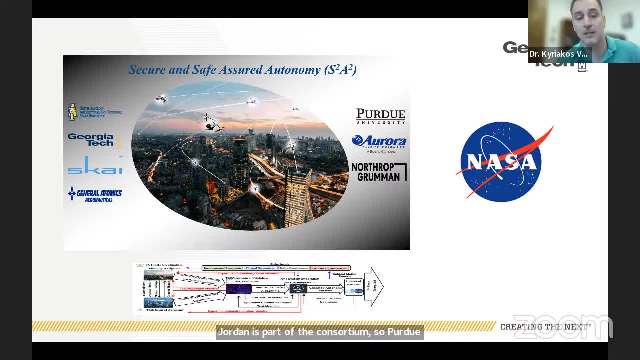 the sky: General Atomic, Northrop Grumman, Aurora, so on and so forth. So we go from perception all the way to verification And we want to make sure that, when we deploy this urban air mobility on the skies, everything is safe and secure. 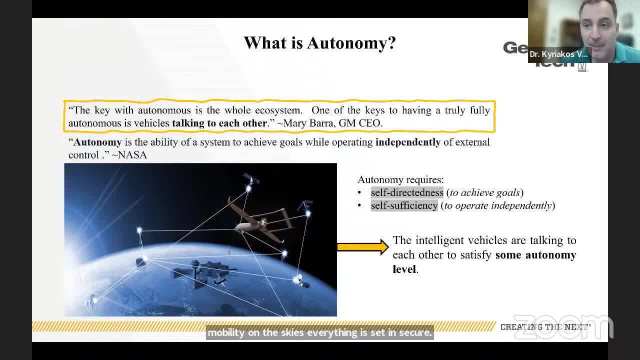 Okay, so let's actually start describing more what is autonomy, or what is autonomy in an engineering glance? okay, So What we want to do is we want to make autonomous the whole ecosystem. okay, So, even if we have multiple components in the system, 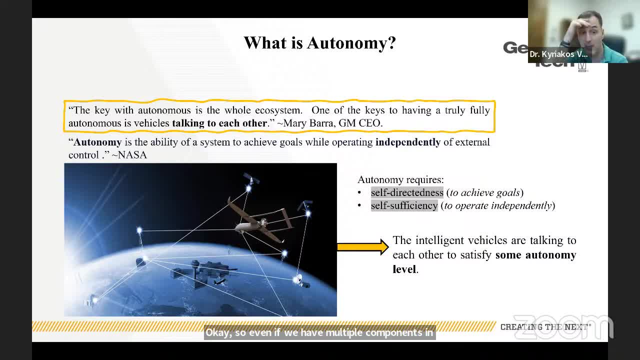 for example, let's say we have multiple planes flying together autonomously, and so on and so forth. So we want to make sure that everything talks to each other in a smart way And, based on that, they make smart decisions. okay, So again, NASA defines autonomy as the ability of a system. 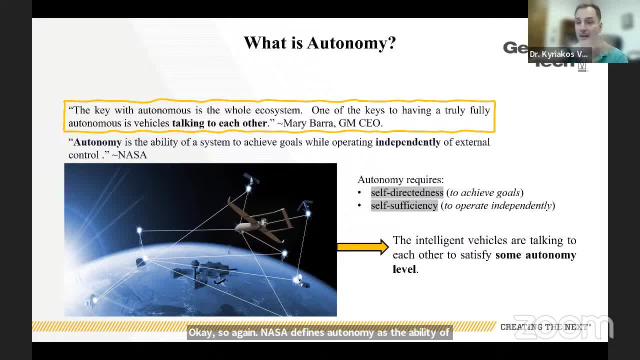 to achieve goals while operating independently of any external control, and I mean external control can either be a human or even a computer sending commands offline. Okay, so autonomy requires self-directedness and self-sufficiency. okay, So what we want to do is we want to achieve goals. 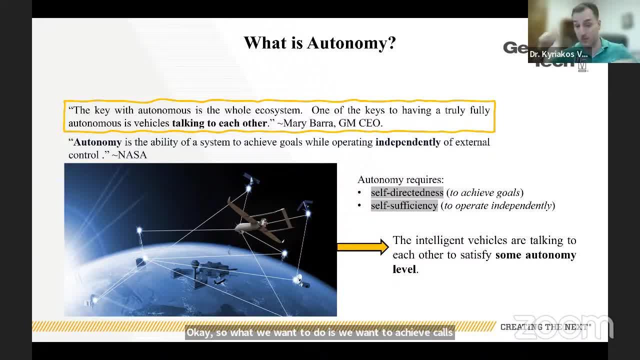 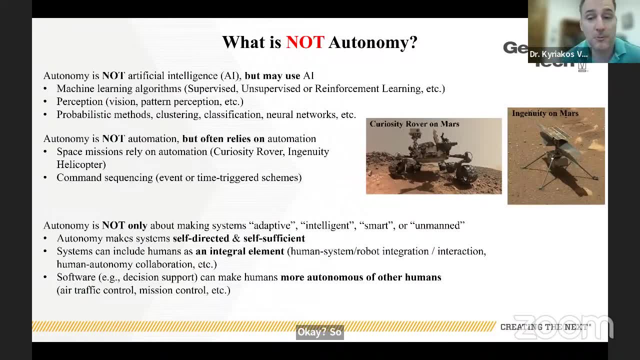 and we want to operate in long-term missions without intervention by the human- okay. So I want also to want to differentiate what is not autonomy- okay. So autonomy is not just AI- okay, Of course, AI is a very useful component of autonomy. 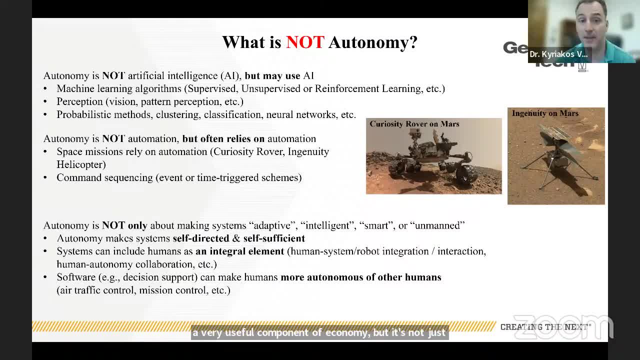 but it's not just AI, okay. So there's many things that actually autonomy comes with. So several machine learning categories. So machine learning is actually under AI and it can be differentiated in three categories. So supervised learning and supervised learning and reinforcement learning- okay. 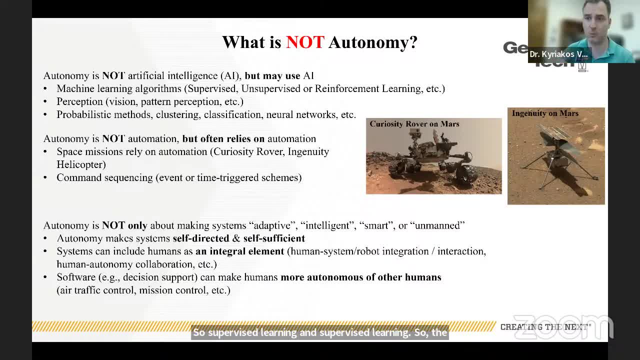 So the perception, just what I can see. okay, How can I perceive my environment? And there's also different other things, like how, for example, let's say, I classify, let's say I drive my Tesla and then I classify this as a stop sign. 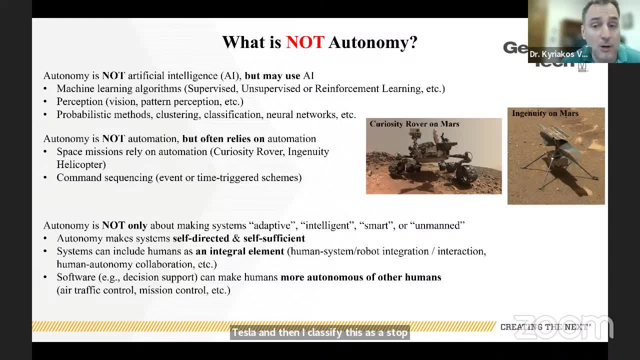 so I have to stop and so on and so forth. So also, autonomy is not automation. So the space missions, they rely on automation. So I'm sure you're familiar with curiosity or with ingenuity, okay. So all these things they rely a lot on automation. 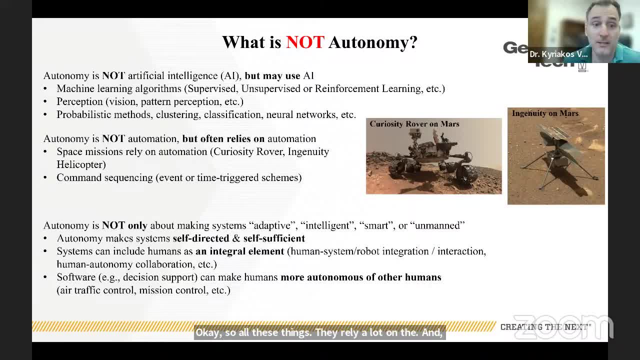 And, of course, autonomy is not always and only about making systems adaptive, intelligent, smart or unmanned- okay, But we want to make them self-sufficient, okay. We want to make them smart- Smart, not in a way that they're just making. 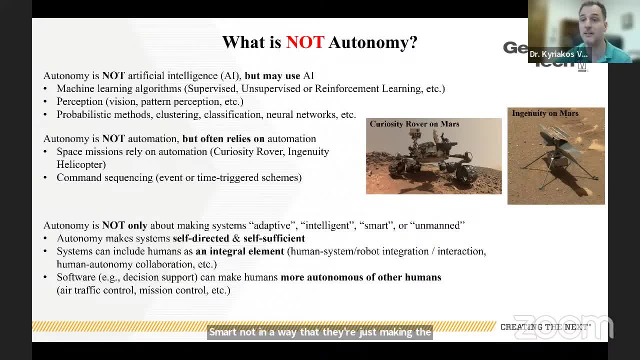 the decision-making, but also they're self-directing themselves, okay, And of course, human is also part of the autonomy right. So humans, they interact with autonomous systems, and so on and so forth. And one actually a very simple scenario. 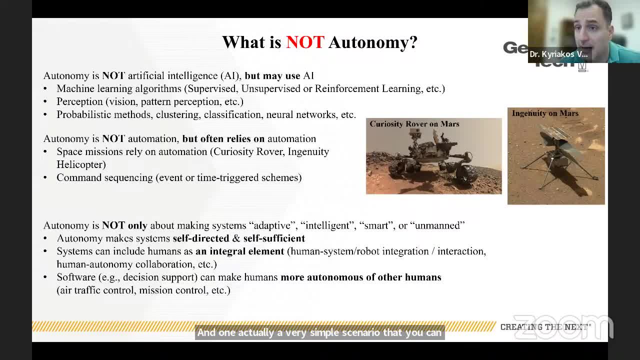 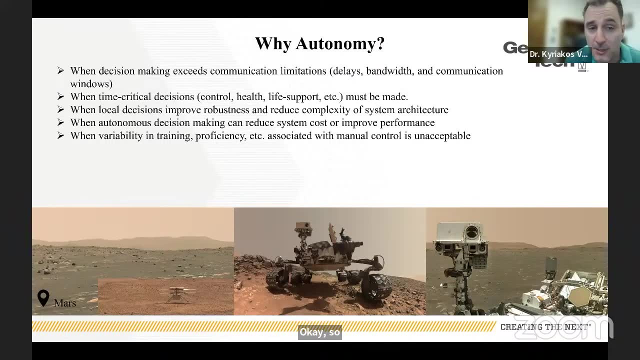 that you can think is about air traffic control, right? So humans, they can interact with decision-makers, that they can happen, from AI to how to reroute aircraft and so on and so forth. Okay, so why we want, and everything actually is going. 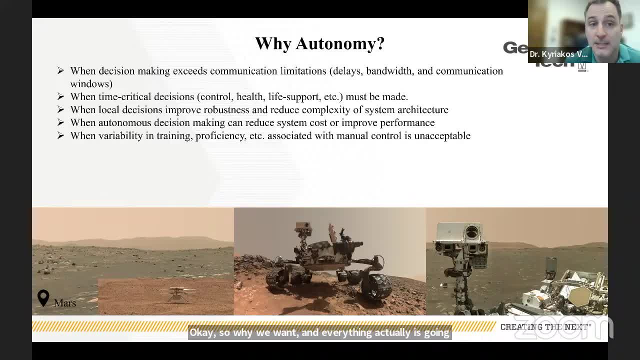 towards the direction of autonomy. why? Because decision-making can exceed communication limitations, and then we have to be smart on what to transmit and when- okay, And also when time-critical decisions must be made. we need to be very smart on what we do. 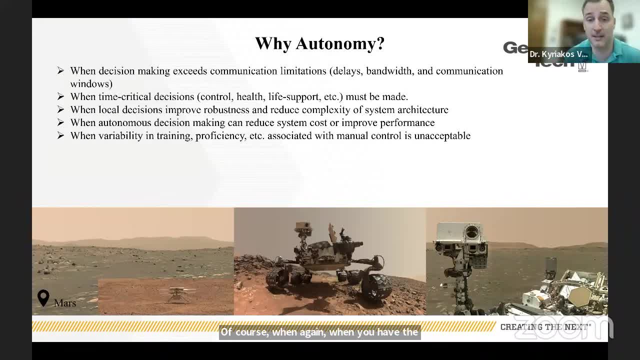 Of course, when- again when- you have the decisions, that they're shared between multiple components, like multiple drones flying together, multiple aircraft flying together, and so on and so forth, So they have to exchange information and then together they have to reduce the complexity. 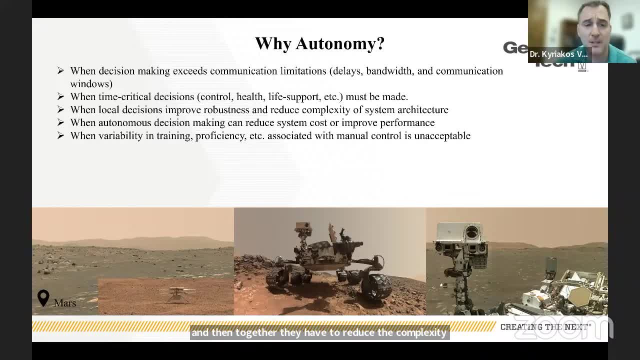 and they have to improve their robustness. So, of course, when we don't have centralized decision-making and we have distributed decision-making, so this actually can make our systems smarter and can make them reduce complications and costs of the system. Of course, when we have autonomy. 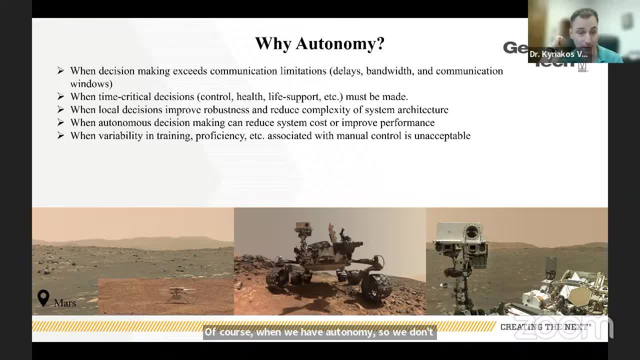 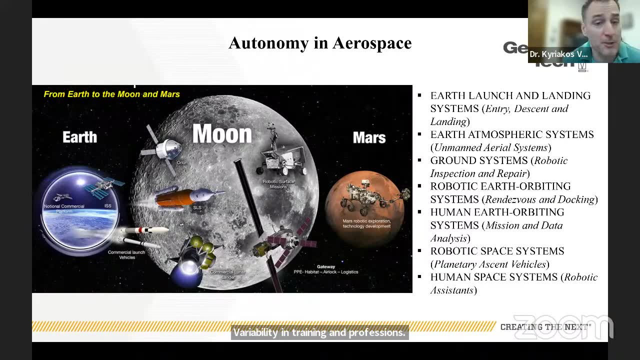 so we don't require or reduce variability. we have good�� lot energy demand control in training and proficiency, Okay. so again, autonomy in airspace goes from the earth towards moon and Mars and so on and so forth. okay. So, for example, 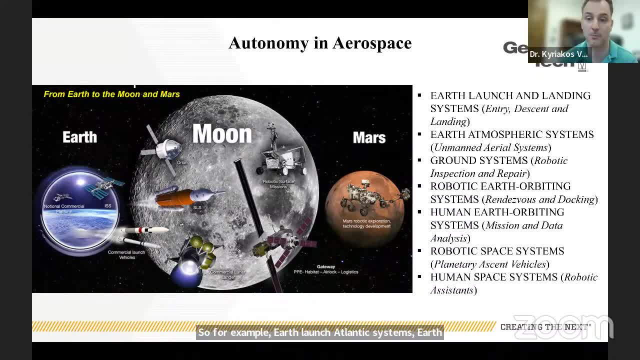 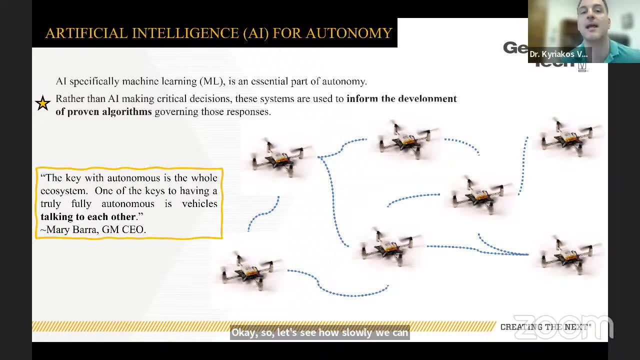 earth launch and landing systems, earth atmospheric systems, ground systems, robotic orther sequences, human earth kuntion systems, robotic space systems and human space systems- All these things. they require as much autonomy as possible. So let's see how slowly we can get into what part of AI makes our system autonomous, okay. 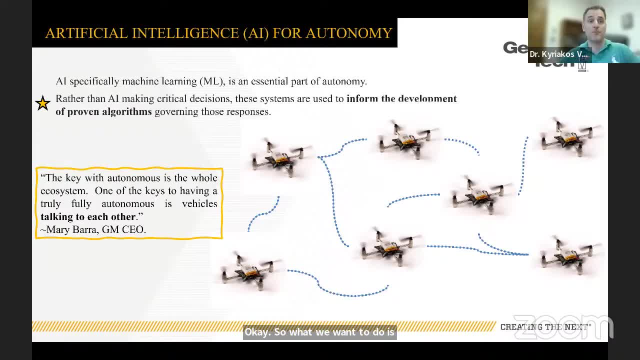 So what we want to do is, instead of just using AI, for example, I think Dan said about ChatGPT, right? So ChatGPT is just a large language model where it is trained and then it will give you some answers, right? 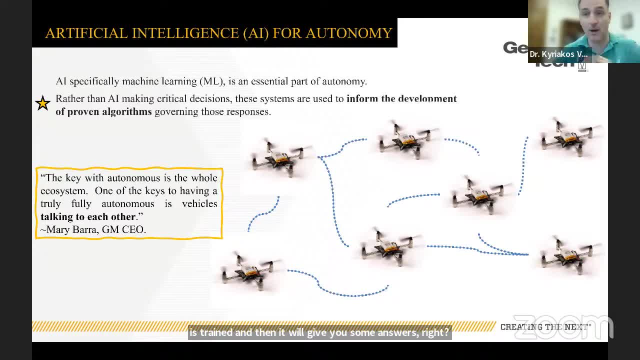 So what we want to do here is we want to have- and all of them are open loop, right? So, in other words, what I mean by open loop is: I don't get feedback from the environment of how good I'm doing, right? 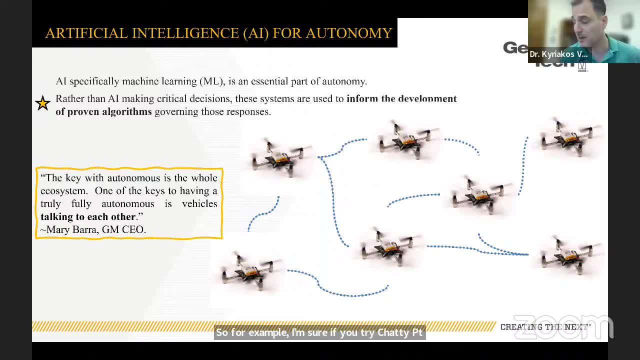 So, for example, I'm sure if you try ChatGPT or OpenPilot- whatever they call it- from Microsoft, you will see that it will give you bad, sometimes bad- things. I mean bad things, I mean very sloppy, but you can always improve them okay. 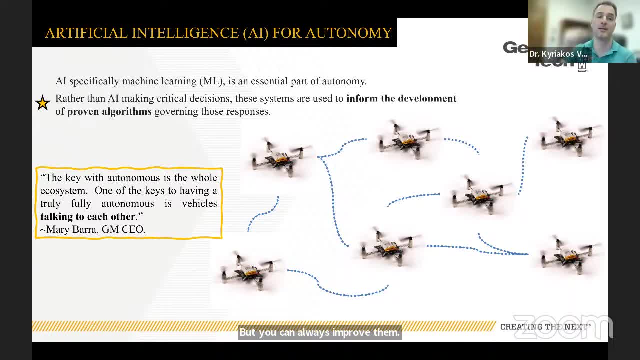 Okay. And By asking: okay, you need to improve it there, you need to improve it there, you need to improve it there, so on and so forth, But we want to have this improvement in a loop that doesn't require this human intervention. okay, 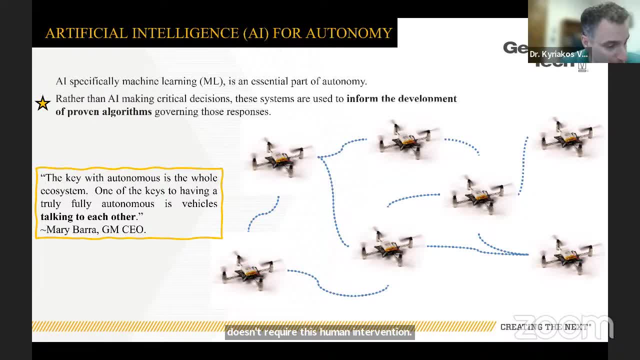 So there is something very popular in control theory, which is my main focus area, where it's called feedback loops. okay, So you can think that I have an aircraft or I have a drone. okay, So I measure things with my environment, from my environment, from my sensors, and based on what? 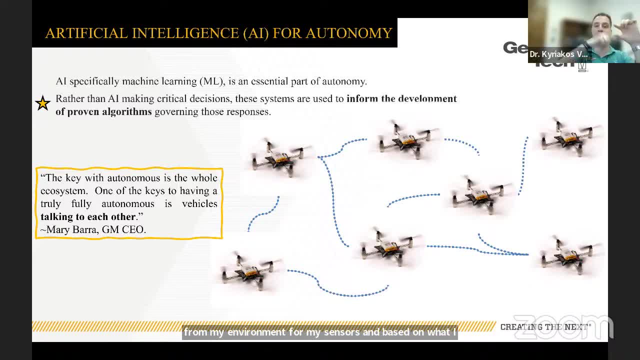 I what measurements I get from my sensors. I can command my actuators of the system. okay, So this is where feedback comes into the game. Okay, So, what we want to do and why. actually, AI is very important in aerospace, and I think 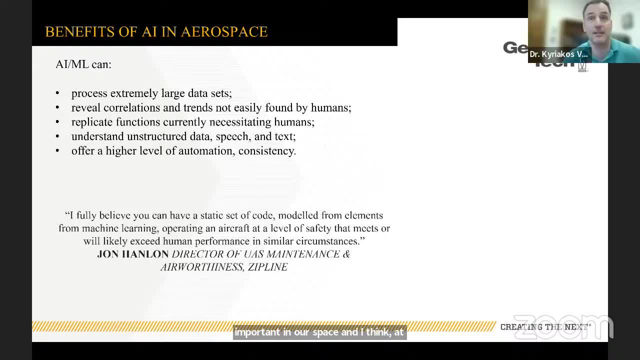 I don't know a single faculty in my department that doesn't work in AI for aerospace is because they can process extremely large data sets. They can find correlations, Correlations and trends that humans they cannot find. they can actually replicate some functions without 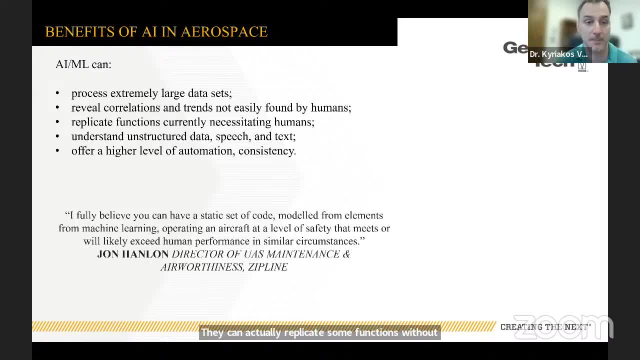 necessitating humans. They can understand data, speech and text, and they can offer a high level of automation and consistency. Okay so, and there's many, many quotes by several people, from any from Sebrek, for example, here from John: 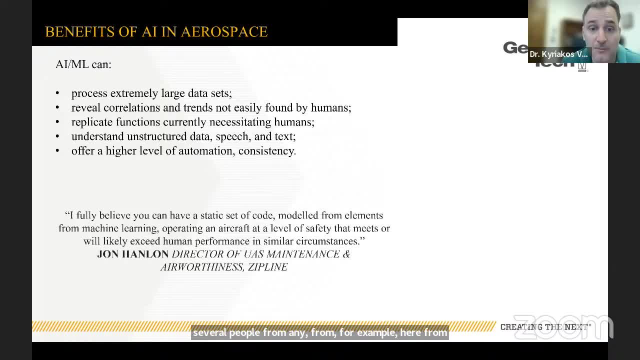 Holland. he said: I truly, I fully believed you can have a static set of code model from elements from machine learning operating an aircraft at the level of safety that meets, or will likely exceed human performances in similar circumstances. okay, so the high impact areas within: 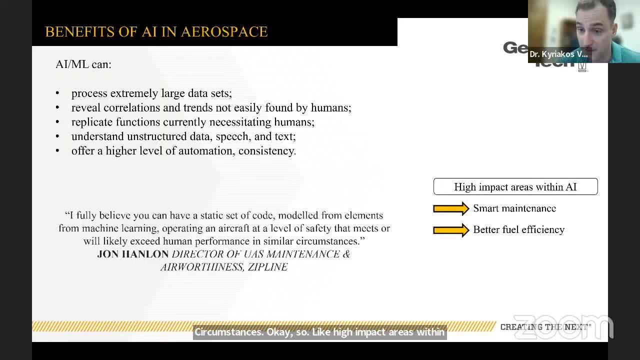 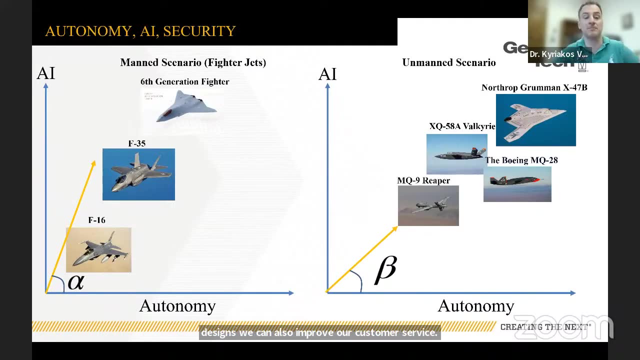 ai are smart maintenance, better fuel efficiency, training and innovative product designs. okay, and of course, if you, if we do innovative product designs, we can also improve our customer service, okay, so now what you see on the left. you know you see two axes right, so one axis is the ai. 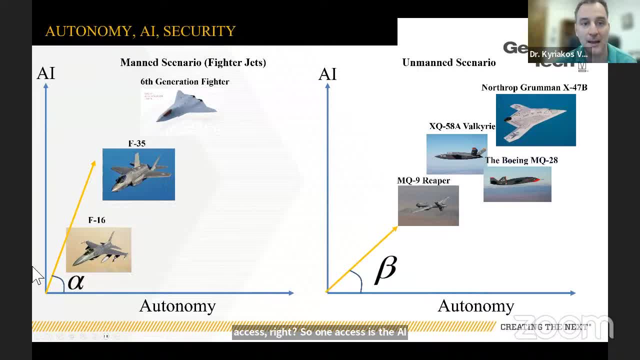 the other axis is the autonomy. so here on the left you can see the manned aircrafts, while on the right you see several unmanned aircrafts, right. so, and then here you see two angles, right, so i try to be very vague here. so you see two angles. you see alpha and beta, okay, so 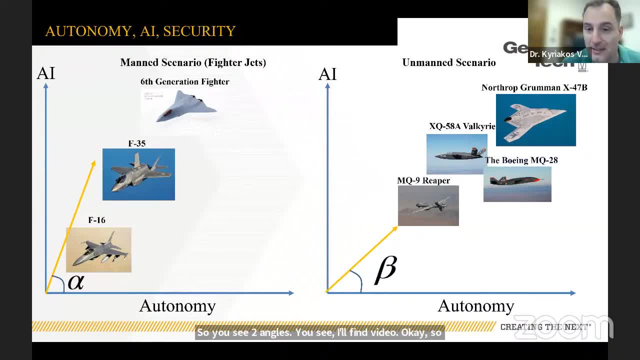 i'm sure that you all can understand that from- i mean from my bad figures- that a is bigger than beta, because the humans, they are better at flying these aircrafts and they know what to do and what not to do. okay, so still, we have lots of work to do in the unmanned scenarios, okay, and i think in 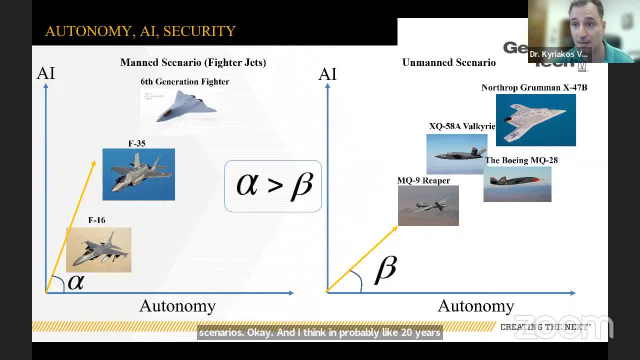 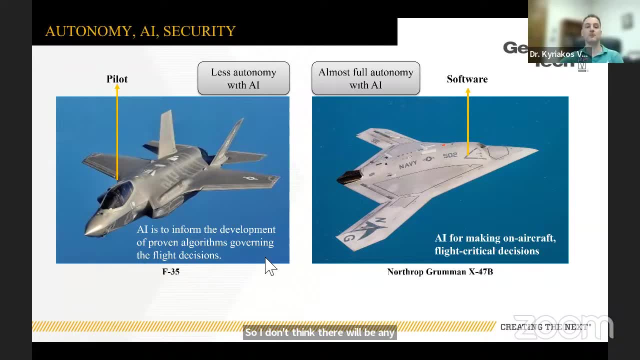 probably like 20 years. everything will happen in the unmanned scenarios, okay, and i think, in in an unmanned play. so i don't think there will be any manned aircrafts anymore, okay. so again, what we want to see here is: so you have a pilot, okay, let's say, in this aircraft, okay. 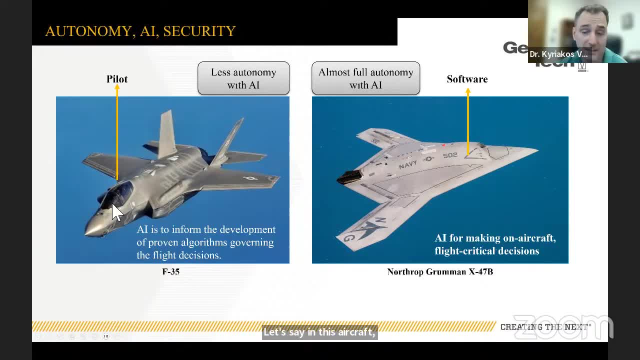 and the pilot makes the decisions right instead on the full autonomous aircrafts. so we don't have a pilot, but we have software right. so the software which actually has to operate like a pilot has to make this on aircraft decisions for flight critical um at times. okay, so nowadays. 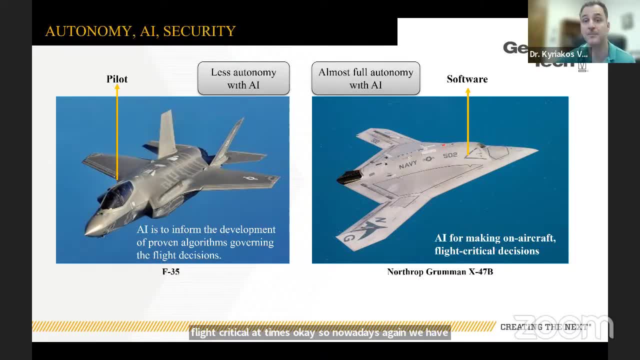 again, we have the pilot. the pilot can make decisions in real time. um, bridging this, uh, this thing now between the pilot and the software is very important, okay. so, again, the pilot is, of course, better trained, can make better decisions, okay, and while the software sometimes can make mistakes, okay. so we need a lot of improvement there. 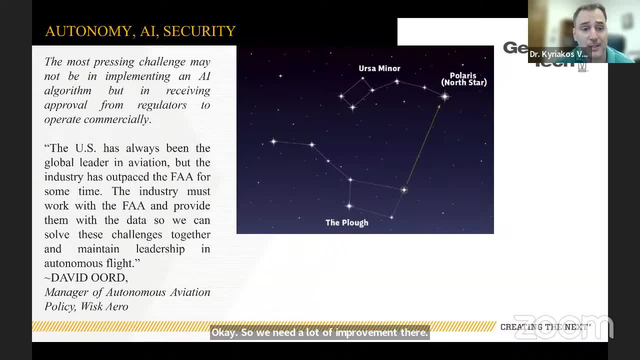 okay. so, um, we discussed a lot about autonomy. okay, we discussed about ai, so, um, i think in in the talk you saw a lot also about security. okay, uh, so why we want to be secure is again, uh, the smarter our, the more vulnerable to adversaries are. okay, so, of course, if you make anything smart, right everything. 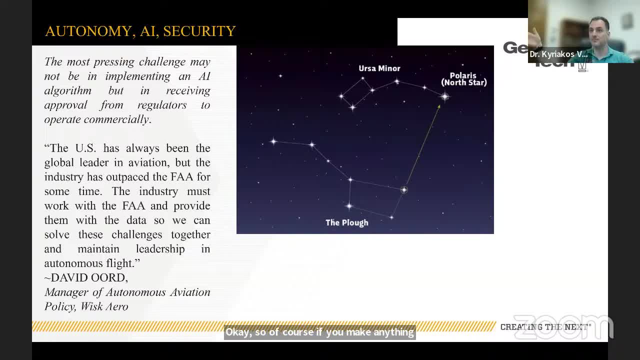 depends on software, so this software have holes and then people can and actually access them and send different commands. so, for example, instead of bumping i don't know one area, bump area b, okay, or things like that, okay, so, uh, so all these things are very important, so and i actually have this. 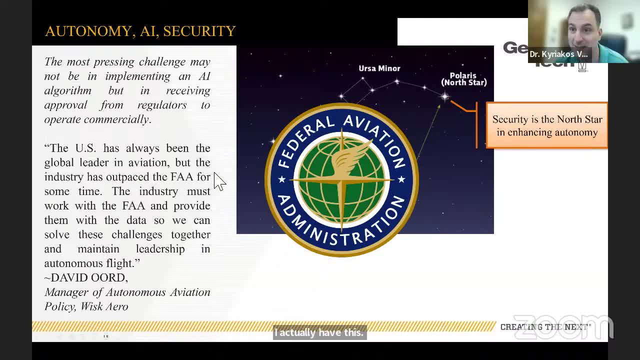 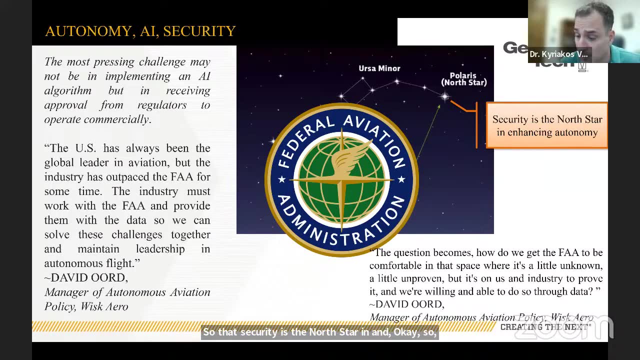 um, this very uh fun uh script here, so that security is the north star in enhancing autonomy. okay, so um again, faa and um needs to work together with uh, with the people working ai, and to make better and more secure algorithms and actually quantify what do we mean by that. 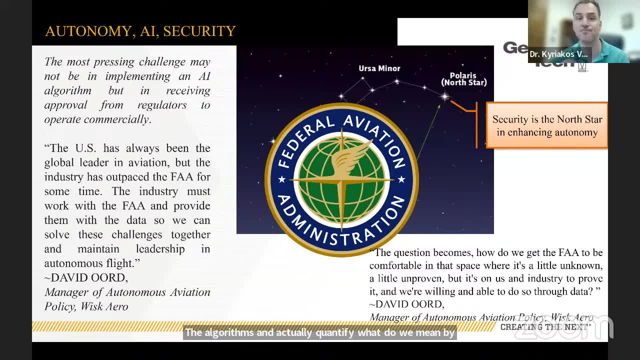 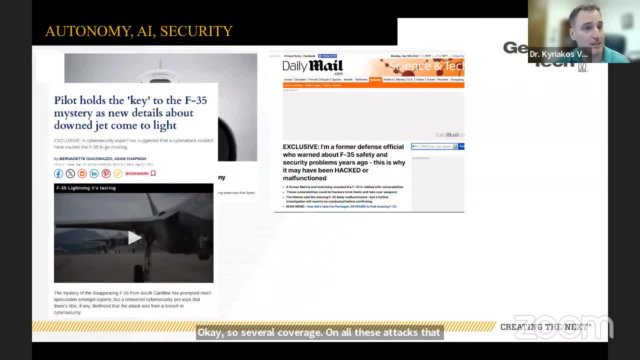 by secure. you'll see pretty soon what i mean by that. okay, so several coverage on on all these attacks that have been everywhere, right? so imagine if these things happen just to pilot aircrafts. imagine what happens in when you have just software piloted aircrafts, right, uh, so i mean. 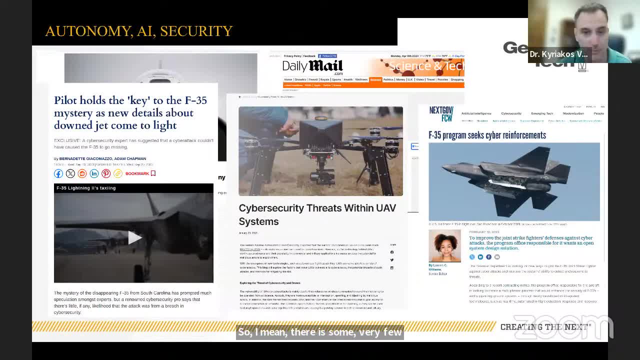 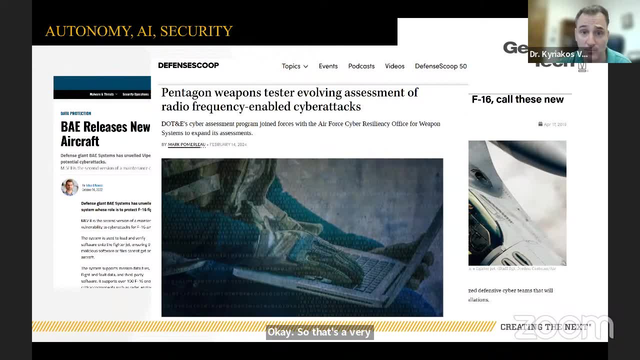 there is some. sure, if you search for them, you'll find lots of news about all these things. okay, um, so that's a very important. so there is uh, um, we have to mitigate these attacks, or even we have to make our controllers- that they are part of this ai- to be very robust to these attacks. okay. 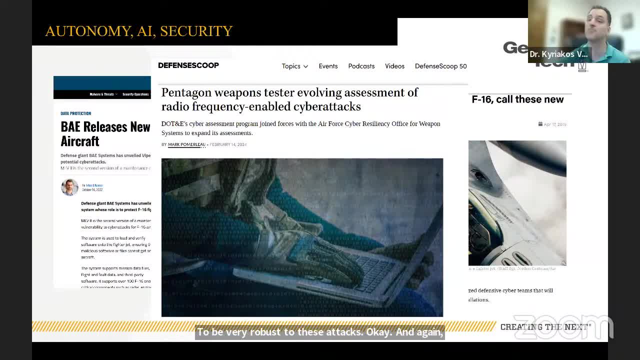 and again there is somebody can say: okay, so the attacks evolve right, even if you find some patches for some other attacks, uh, the attackers can find new attacks. okay, so, because they have through time, so you'll see what are the, what we can do for those things. okay, so, um, some thoughts. 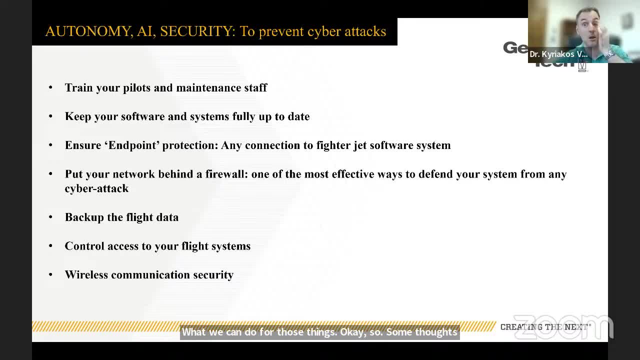 on what we can do to prevent cyber attacks. okay, so, of course, train our pilots and maintenance staff. okay, keep our software and systems fully up to date. again, these are just suggestions for uh, for these things. maybe there are other things. ensure endpoint protection: okay, so any connection? 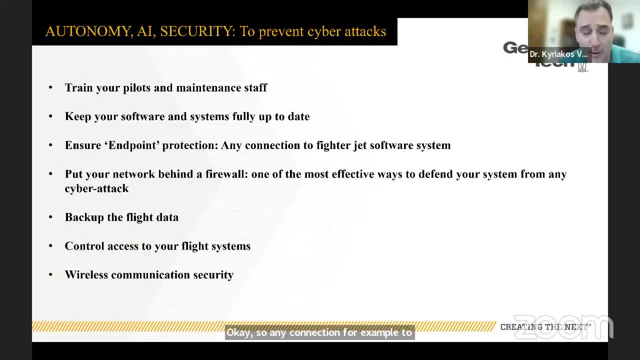 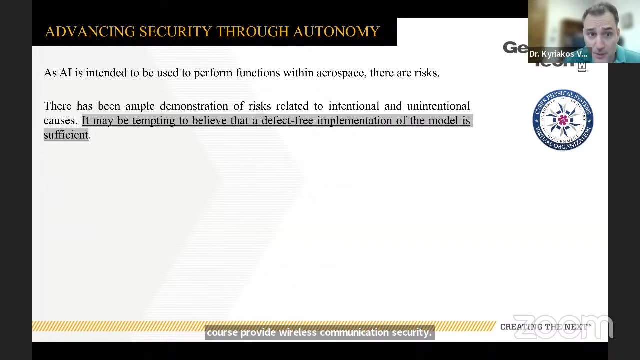 for example, to find a software system, use firewall, uh, backup, flight data control, who has access to your flight systems and, of course, provide wireless communication security. okay, so, um, of course, as i said, nothing is perfect. right, there might be doors for adversaries to attack and make our autonomous system, or even 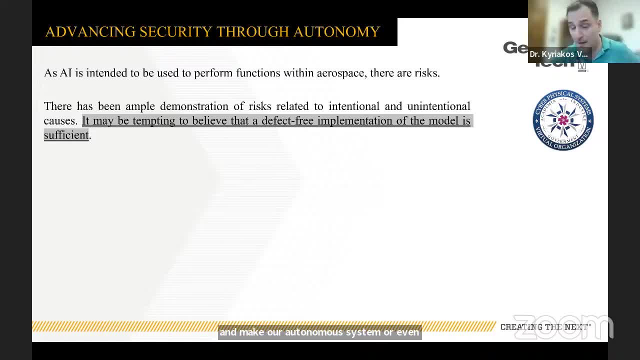 as you saw in the news, our fighter, uh, our pilot, um aircraft systems like f-35 to have to be vulnerable to attacks? right, okay so, um, it is twofold: okay so uh, the environment in which the i, the ai model, is built and the data set used to train the ai model. okay, so, these are the source of safety risks. 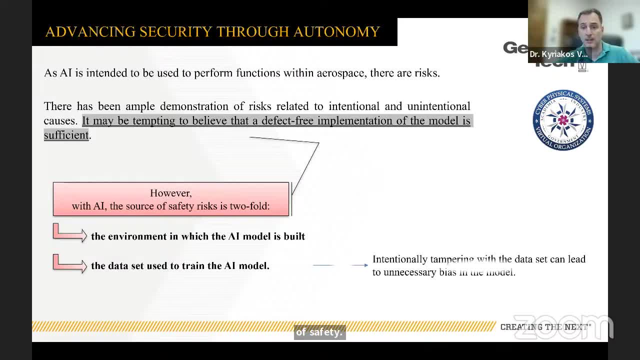 again. so every time, uh, some adversary wants to do something, it can change the data and these two things and then it can make our, our system to do whatever they want. so, again, these are very important. okay, again, we can do, uh, impacting the environment. of course they want to be. 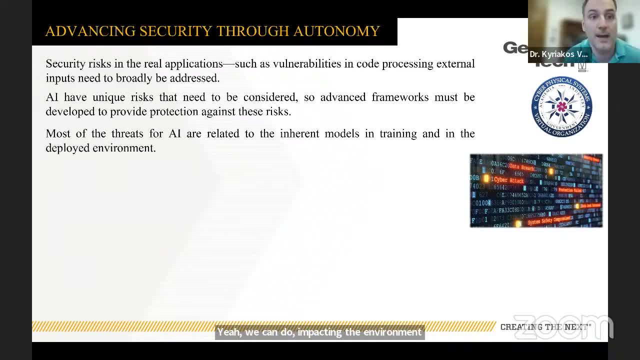 skewed from its purpose and so on, so forth. okay, so, um, what we can do now is we can do the following: okay, so we have very unique risks that need to be considered, so several advanced frameworks must be developed to provide protection against this, these risks. okay, so there are two things we can do: either to to train the people, uh, to work together. 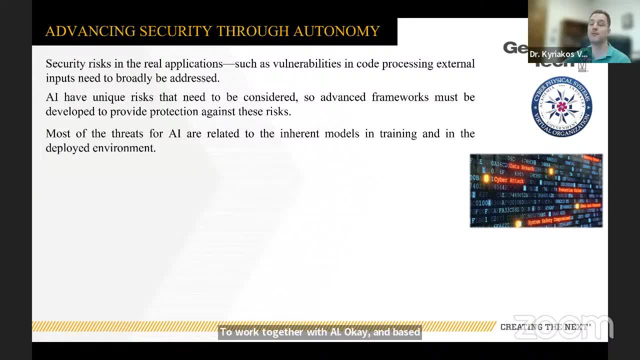 with ai. okay, and based on that, try to see. for example, we have a project, another project with the department of defense, where we want to train human analysts, alongside ai, to predict attacks that can happen in drones, for example, flying over iraq. okay, so we, we want. 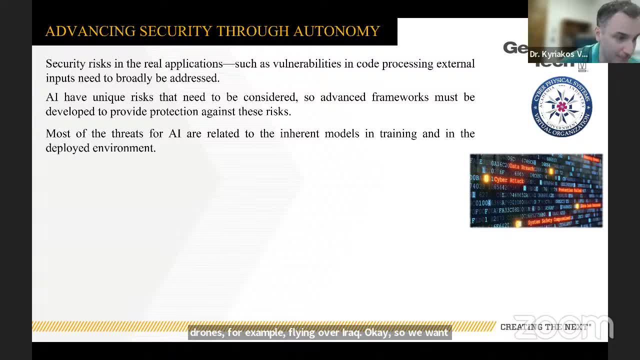 the analyst to be trained together with this ai to differentiate attacks, for examples, from a win cast. okay, so is it an attack or is that the windcast or something happening there? okay, so the most known ai threads are model logic thread, model by passing and, of course, all these things. 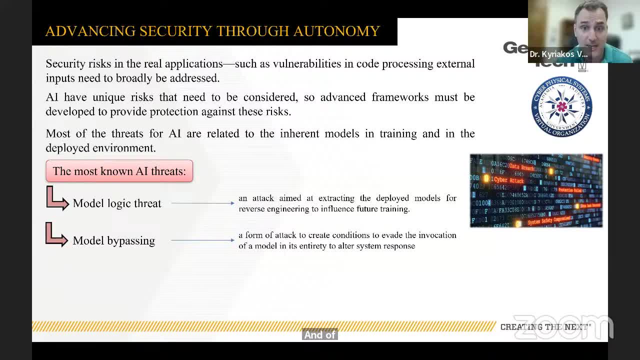 i mean i can explain to you from, for example, the model logic thread: is a threat that literally, that within the model of a threat, if you are playing a game that is going to be a fraud, that a threat is model locked in. threat is an attack aimed at extracting the deployed models for reverse. 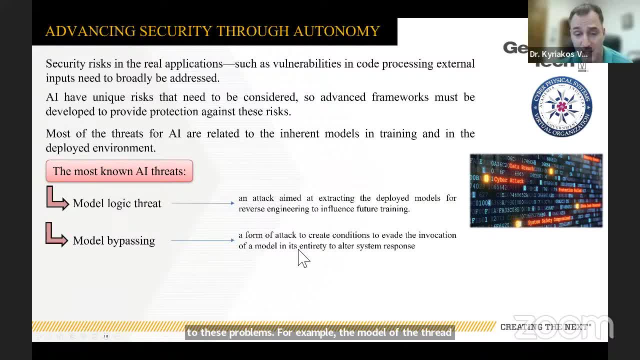 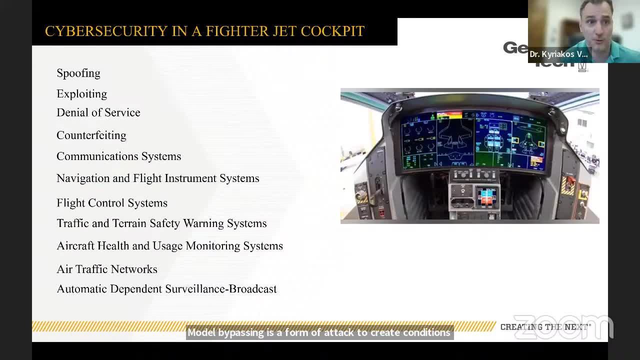 engineering to influence future training. Model bypassing is a form of attack to create conditions to evade the innovation of the model in its entirety, to alter system response and so on and so forth. Okay, so, of course, in a fighter jet cockpit. okay, so people can do spoofing, exploiting denial of. 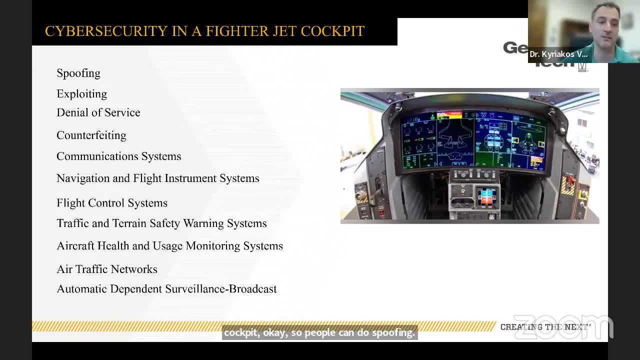 service counterfeiting. they can change the communication systems, the navigation and flight instrument systems, the flight control system- which is actually something that we heavily work on- the traffic and terrain safety warning systems, and so on and so forth. Okay, so these are the doors. 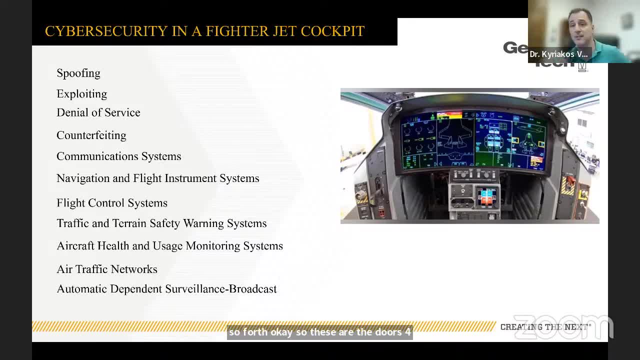 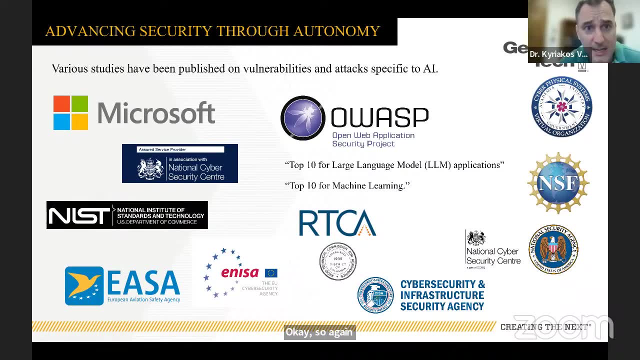 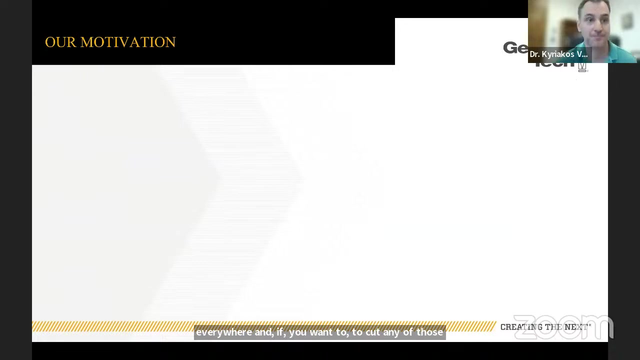 for an adversary to actually change what they do during a flight. Okay, so again, there are several studies on run-of-the-mill attacks specific to AI. Of course, they're everywhere, and if you want to have any of those, just let me know in an email. I will send you any of those. Okay, so what we want? 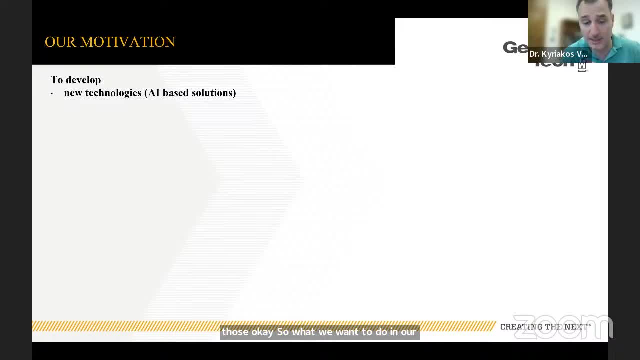 to do in our lab and also in the project. actually, that Dan said from NASA is we develop these new technologies that are, of course, they're AI-based- okay, and they're secure, and they learn on the fly without any pre-training- okay. So, of course, in order for us to do that, we have to consider: 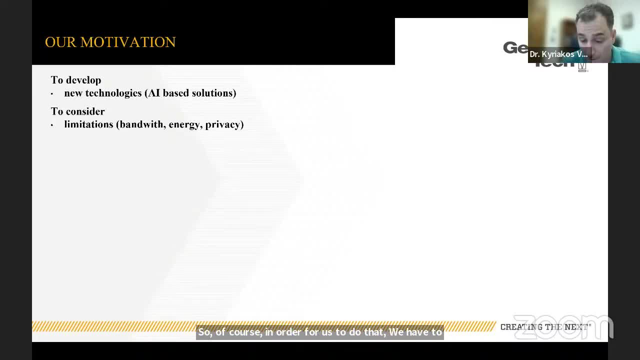 limitations. What do I mean by limitations? So, whenever you are communicating, you have bandwidth, energy and privacy. communications- right. So the more you transmit information, the more vulnerable you are to specific to any type of attacks. right So, the less the least. 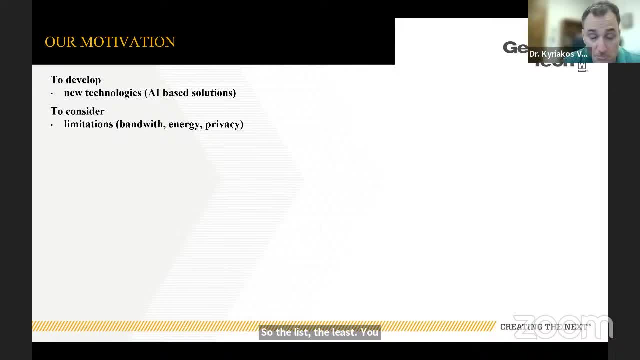 you transfer anything, so I mean the least vulnerable- you will be Okay. so our lab works together to bring together these three things: autonomy, security and coherent data integration. okay, and we have shown that to aircrafts, ground vehicles, underwater vehicles and other. 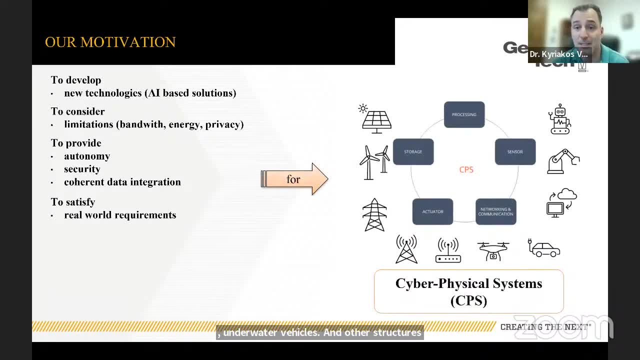 structures. Okay, so all these things that you saw here, they can actually come together on something that we will call as a cyber-physical system. okay, So you can consider that an aircraft is a cyber-physical system. okay, because we have a cyber-physical system, that is a cyber-physical system. 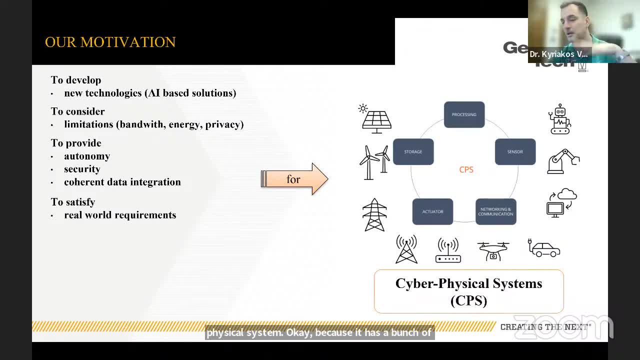 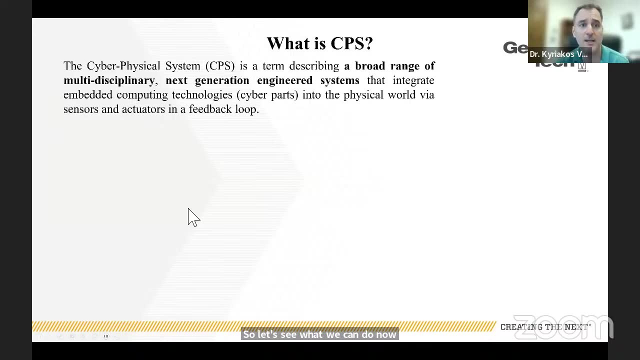 it has a bunch of sensors, actuators, it has processing units and so on, so forth, so we can call it as a cyber physical system, okay so. so let's see what we can do now. again, this is what i just said. okay, so, a cyber physical system is something that gets cyber. 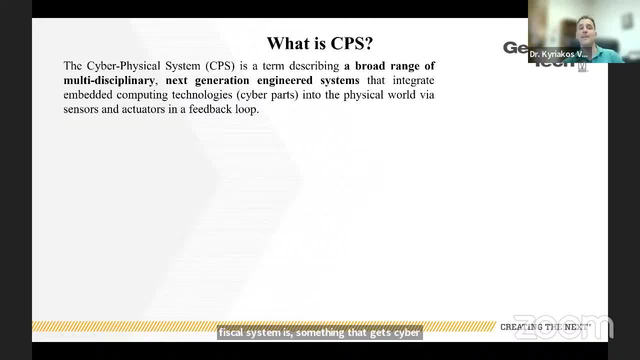 parts which, for example, you can think about any embedded computers okay- into the physical world via sensor and actuators, okay. so again, i want you to see that everything that we will do here is because we are in safety critical applications like aircraft and so on, so forth. we have to be 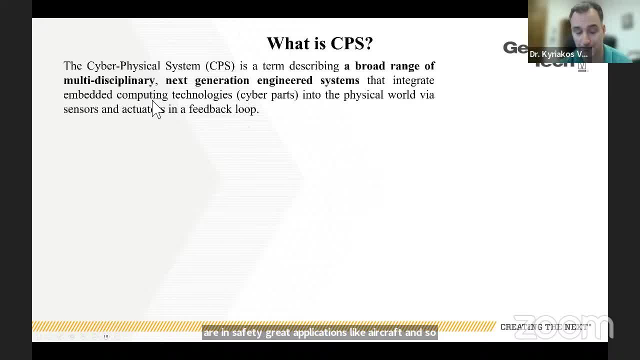 guaranteed to be stable and we will use everything in a feedback loop. okay, so i'm sure you have seen the problems of robustness and stability of train with ai, because they're all of them. they're open loop, so that they're getting sensing from the environment, and they work only on cases that they have been trained with. so what? 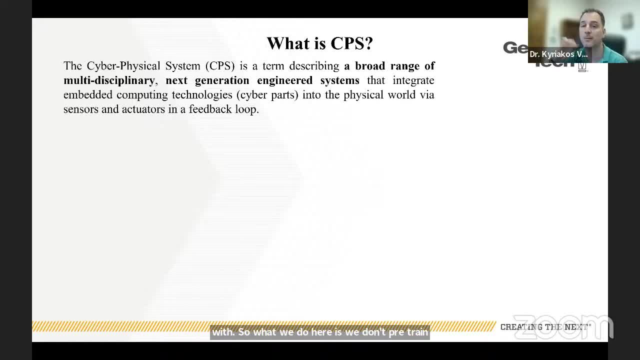 we do here is: we don't pre-train, but it's a more of a plug and play framework that eventually make all the systems optimal, robust and stable. okay, so again, you can think that here is your sensing and actuators. right, so you can think that. 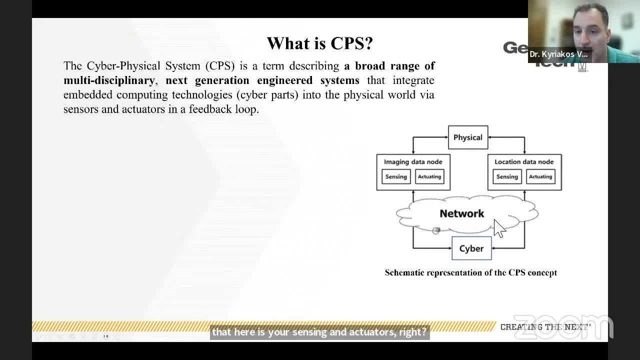 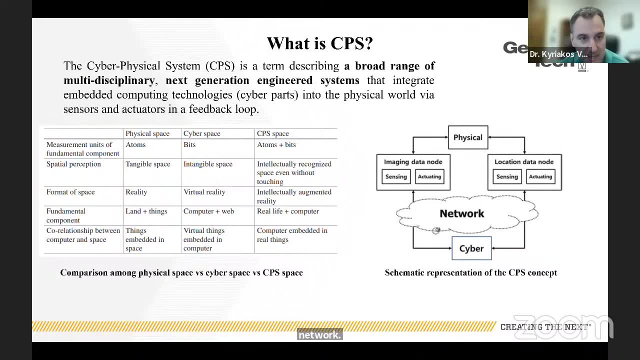 this. kids are involved in this and this is how i should do it. okay, so if you have a precise product control, you need to do that. you need to have a good perception. okay, the first step is you need to enter your perception- okay, this is where i am, and then you communicate through a network. 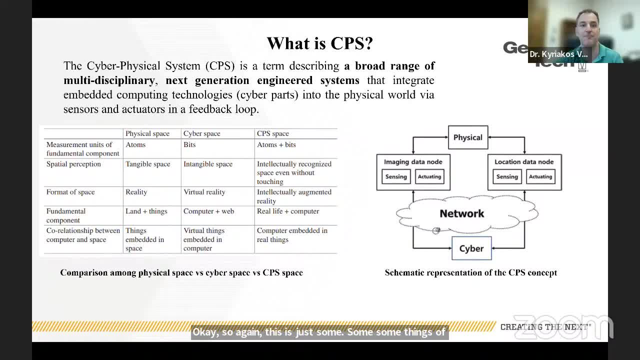 okay, so again, this is just some, uh, some some things of what is physical space, what's cyber space and what's a cyber physical space. okay, so, again, this is- don't worry too much about it. okay so, but what i wanted to pay attention is for those of you who are familiar with embedded systems: 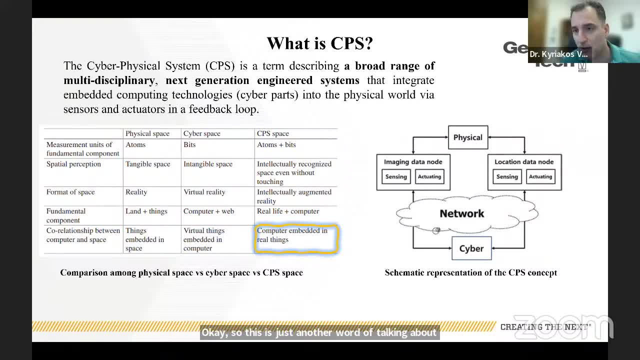 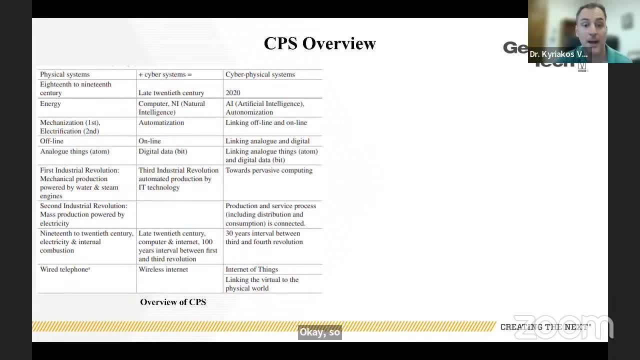 this is just another word of talking about it, but everything is through a network. Okay, so we're right on time. Okay, so what again? what we want to do? and then you see on the left, you see different applications, right, And you see how they evolve. Okay, so you have the AI. 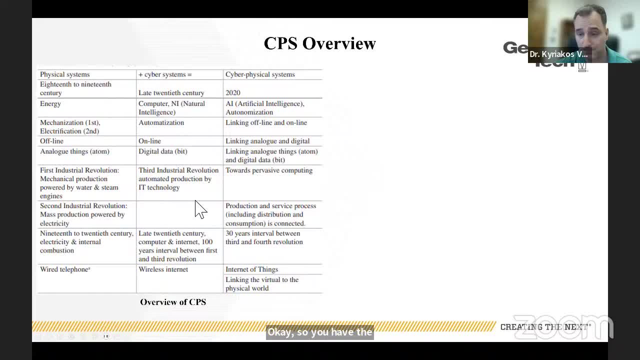 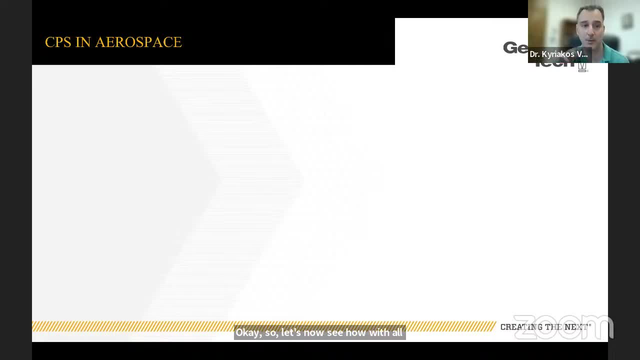 automatization, online, offline, so on and so forth. Okay, so let's now see how all these CPS approaches cyber-physical systems. they can be used in aerospace, Okay. so what we want to do is we're going to bridge the real world with the virtual world, okay, through the sensor network. 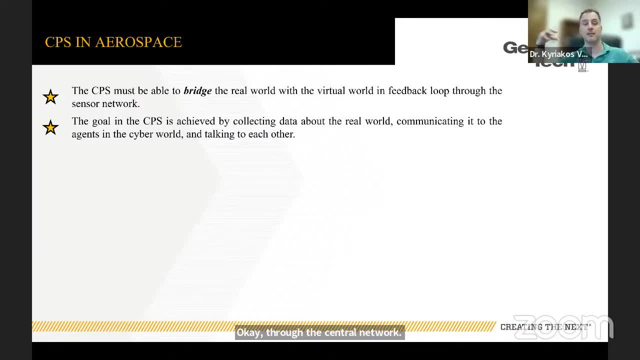 We want to achieve, to collect data, communicate between different agents and then, for example, let's say again, you have multiple aircrafts flying around. they have to exchange information. we have to see what information from all these things is useful and whatnot, and based on that, 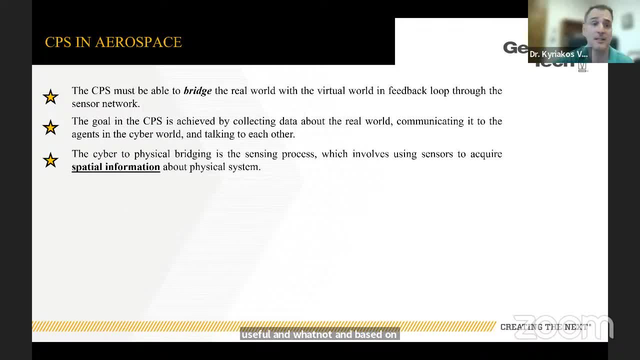 make these smart decisions. So, again, what we want to do is, in order for the cyber to be briefed to the physical world, okay, we need to acquire sparse information about the physical system Again, what I'm measuring, when I'm measuring, so, velocity sensor, GPS and so on. 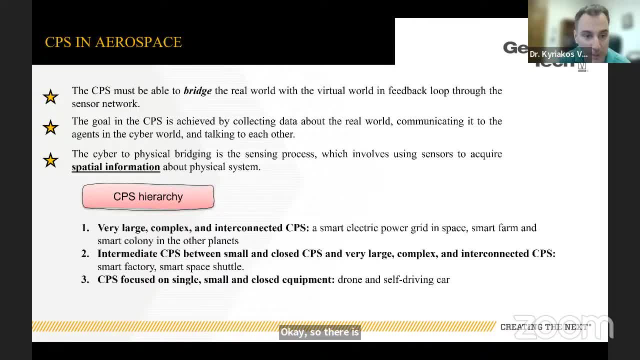 Okay so there is something that we will call as a CPS hierarchy. Okay so, for example, let's say, you can have a very, very large, complex, interconnected cyber-physical systems which can be electric power grid in space, a smart farm, a smart colony in the other. 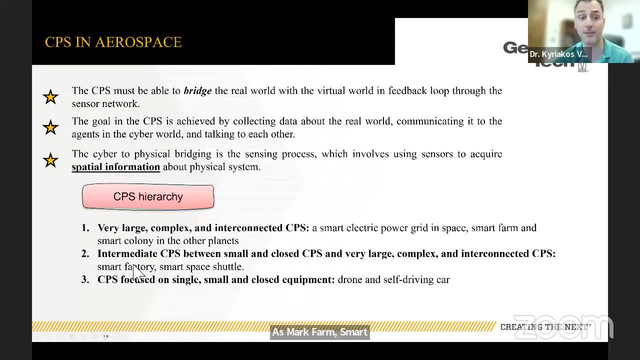 planets, and so on and so forth. You can also have an intermediate, CPS, and which are, for example, a smart factory, a smart space outpost, and so on and so forth. Or you can have a small one, okay, which is, let's say, a drone or a self-driving car, Okay, so all these things they go from. 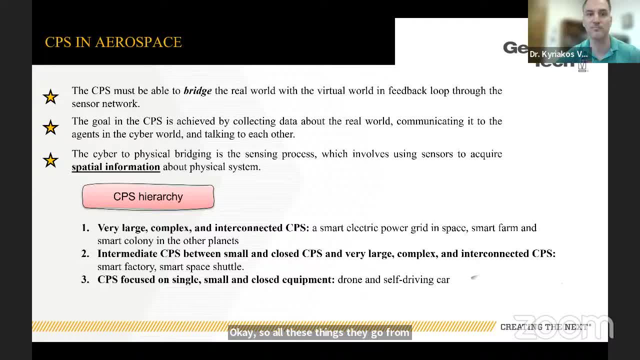 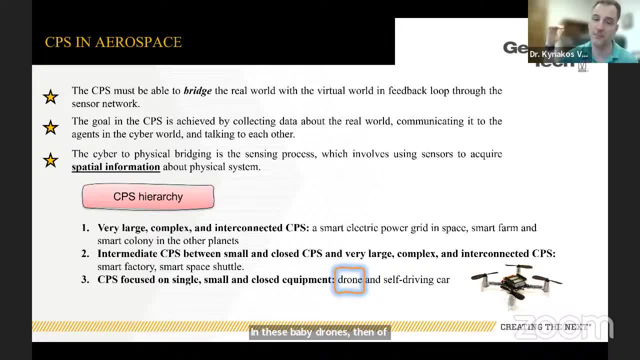 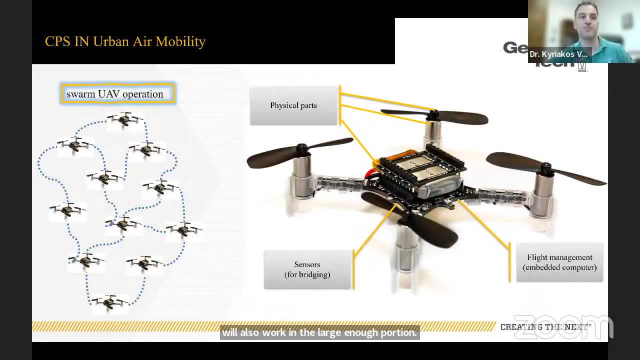 in these baby drones, then, of course, if you make it to a bigger, that you have better and faster computers, everything will be easier, right? So everything that works in these baby drones, then it will also work in the larger ones, of course. Okay, so again, you can imagine that. 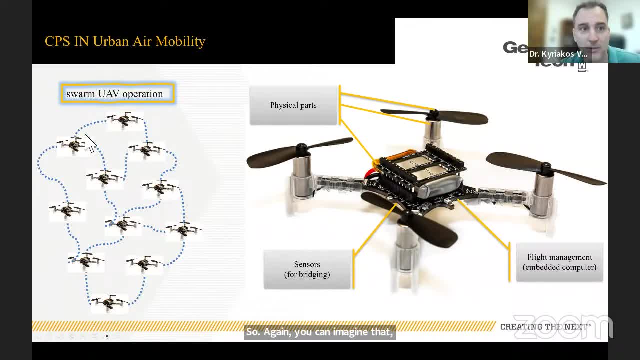 instead of having these baby drones, you have actually, for example, large flying cars. Okay, they all navigate around. okay, they have humans, they have different things with them and they want to navigate around the buildings and they don't want to crash to each other. 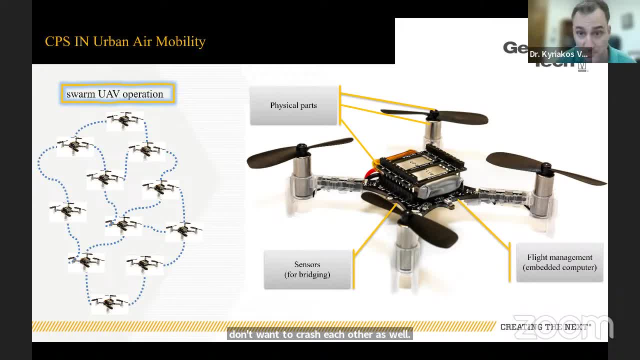 as well. they don't want to crash to the buildings, right? So in this baby drone, the manufacturer called it the CrazyFly, so you see the physical parts, right So, the physical parts, and you also see the sensors where you can measure what you measure. okay, So again. 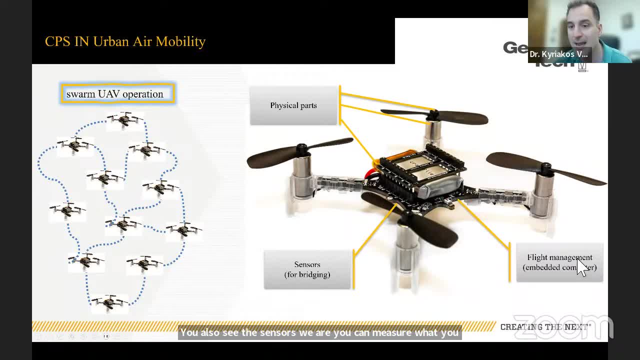 the sensors are bridging the physical with the cyber part, okay, And all the flight management is happening inside this embedded computer, that's inside this bot here, okay, Okay. so again, remember before I said that one of the keys to having a truly fully autonomous 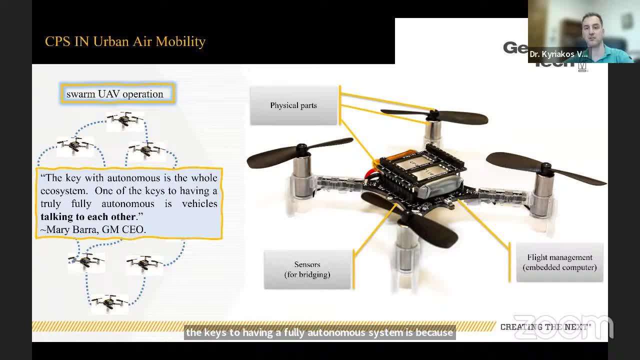 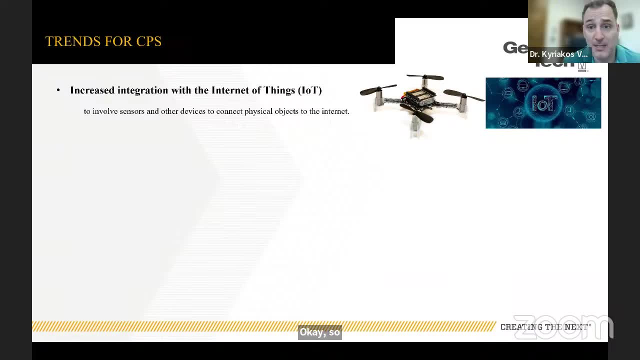 system is vehicles talking to each other in a smart way and making smart decisions on the flight. Okay, So again the trends for the cyber physical systems. they go from integrators with Internet of Things. right, So Internet of Things can also be integrated with through binary mobility. 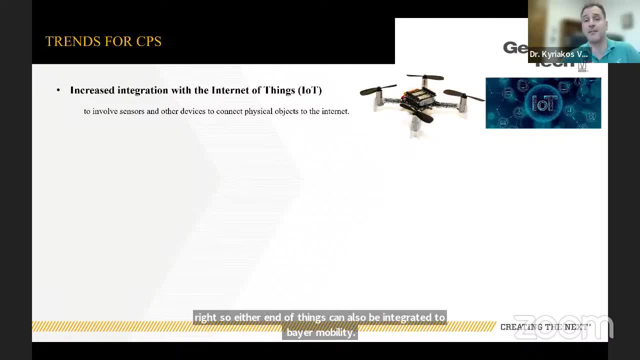 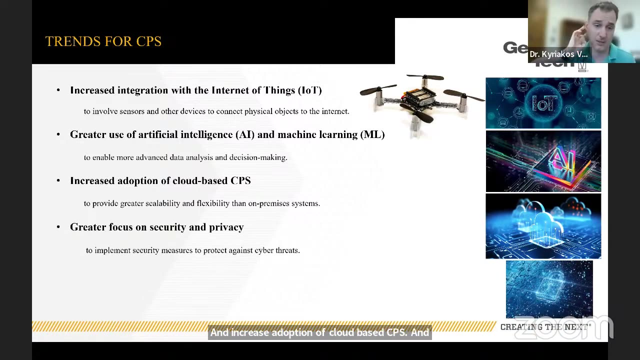 service space will be integrated with Internet of Things and everything will be in a 6G situation, if you can say that. Okay, Again, greater use of AI and machine learning and increased adoption of cloud based CPS- And, yeah, this actually. 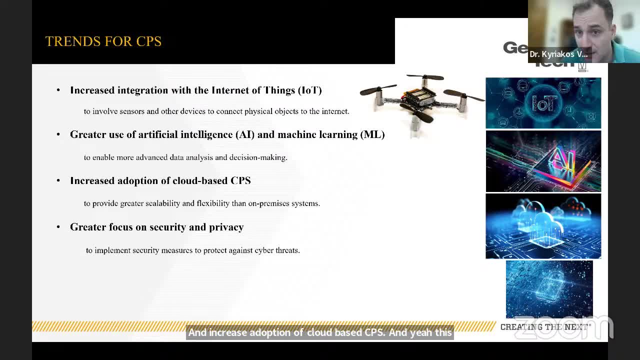 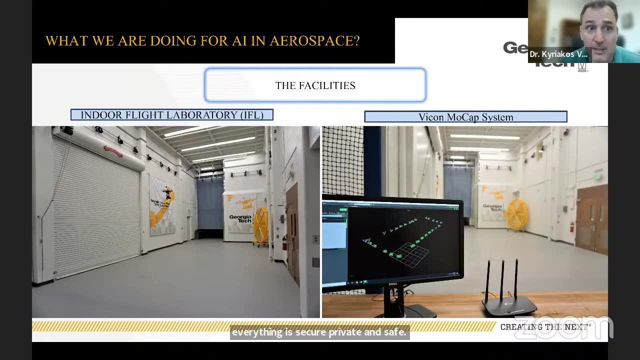 goes back to create a focus on security and privacy. okay, so again, the smarter the systems, the more vulnerable to attacks and the more vulnerable to um to expose data. so that's why we have to make sure that everything is secure, private and safe. okay, so now? uh, let me talk. 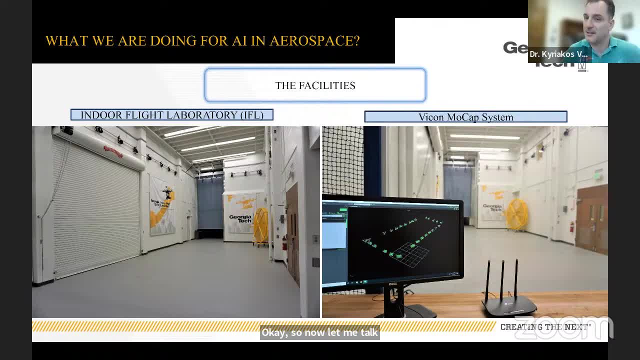 briefly about how do we test these things in a lab environment. okay, so what you see here is you can see our indoor flight facility lab at georgia tech. okay, so we have two rooms. okay, so here around you can see we have infrared cameras. so these infrared cameras, they will measure the 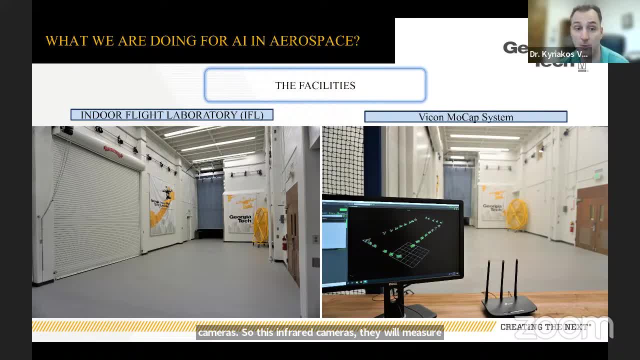 position of of the drones. okay, so this is a facility that we fly. also, here you can see a fan, so this fan will create some disturbances into our drones and then we will be able to see if we're a bus to such disturbances. so So, in a situation that this flies outside, 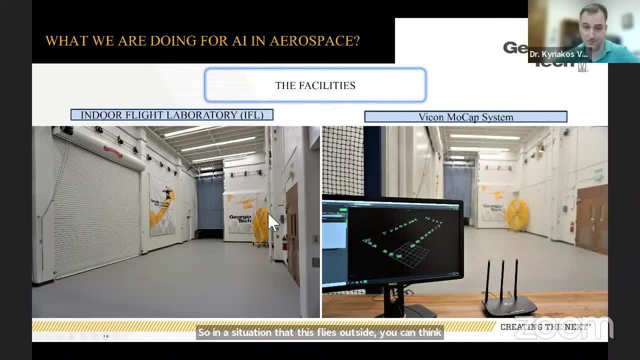 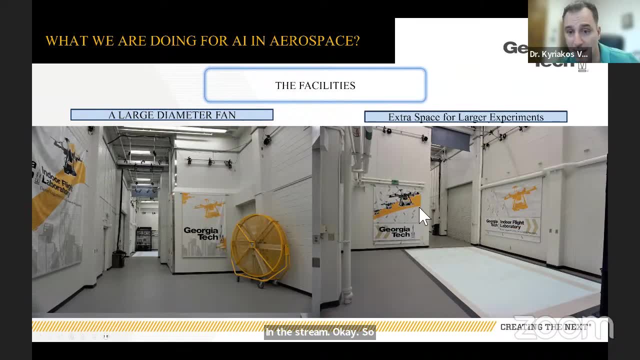 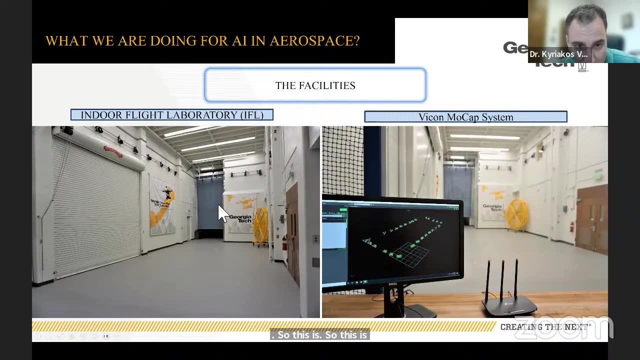 you can think this is just a windcast that will be introduced in the stream. Okay, so again, this is just the other area. So you remember that this is so this is and not the other room, that you can fly towards the other room. 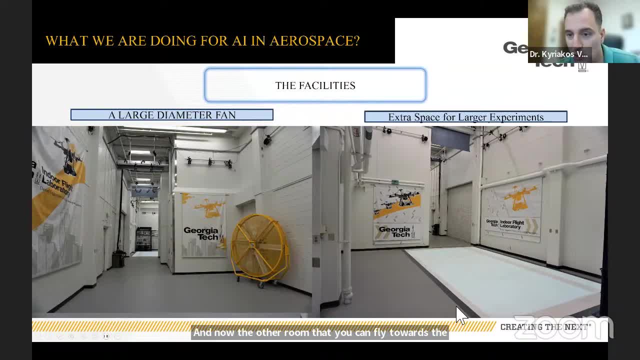 And then here in the other room we have a projector, okay, that projects on the ground, And this projector can actually do different buildings, It can do different areas, So we can actually create artificial or virtual obstacles. Okay, so one very, as I said, 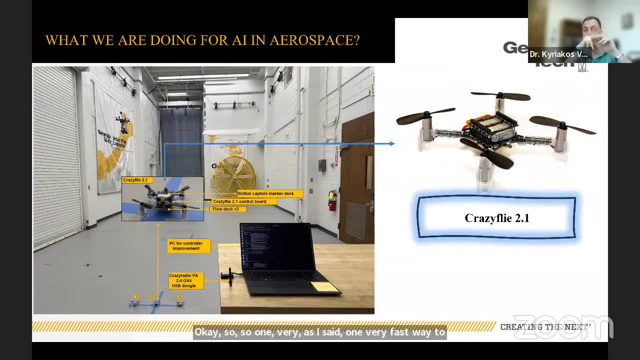 one very fast way to test our algorithms in aerospace is to use these baby drones which, as I said, they're crazy flies. So here you see, a setting of these crazy flies, where you can see- you can see that we have the flow deck. 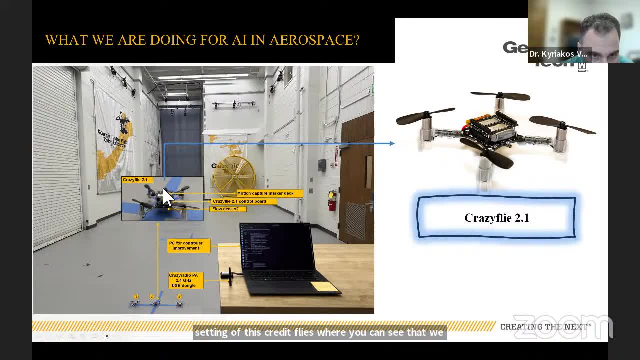 we have the control board and then here you see some little balls. okay, So these balls, they actually are markers, where these cameras will make sure that they're marked and give you a positioning on the ground. okay, So again, these markers are just to be positioned. 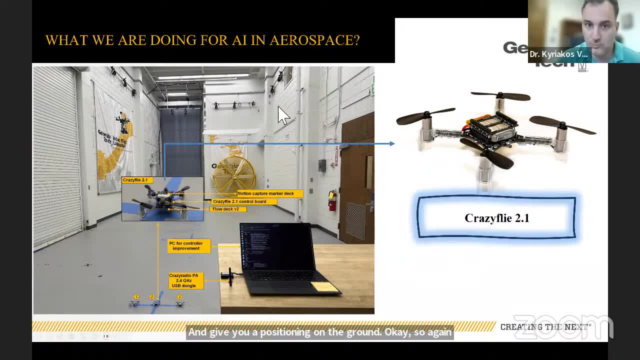 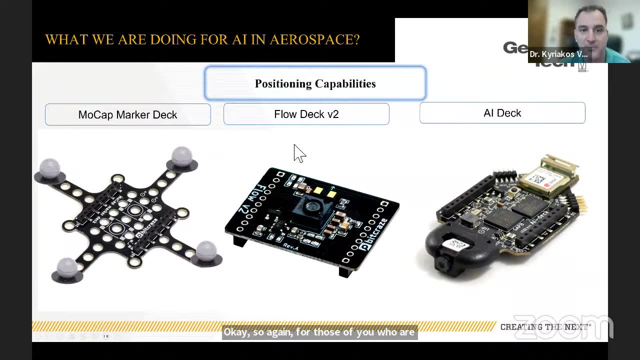 by the cameras. Okay, so again for those of you who are also interested in how this can be built right, So we have a marker deck, a flow deck, an AI deck, okay, So you can think all these things are just having sensor actuators. 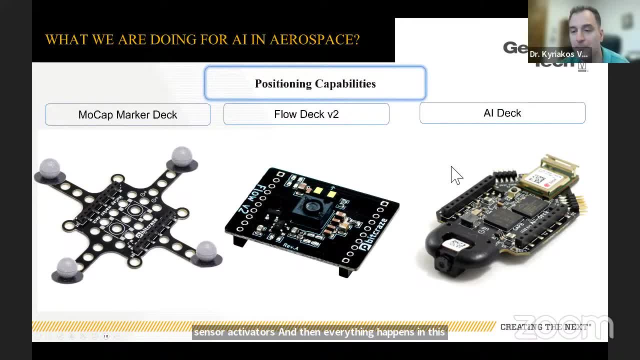 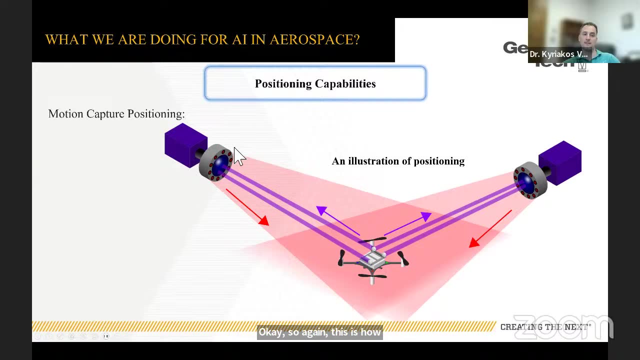 And then everything happens in this small board. So the AI that we test for our NASA project actually can fit in this little baby board here. Okay, so again, this is how the motion capture positioning works. okay, So you have different, you have different. 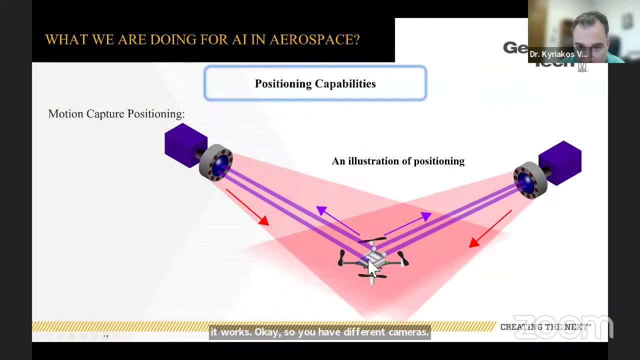 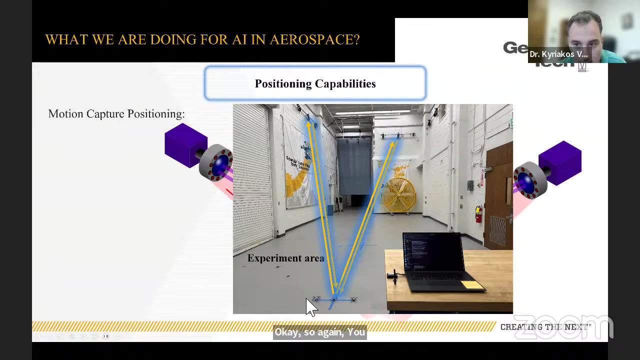 you have different cameras. okay, So you remember I had these little balls here. okay, So these little balls will tell me where exactly I am on the space. Okay, so again you can see. here we have three crazy flies: the cameras. 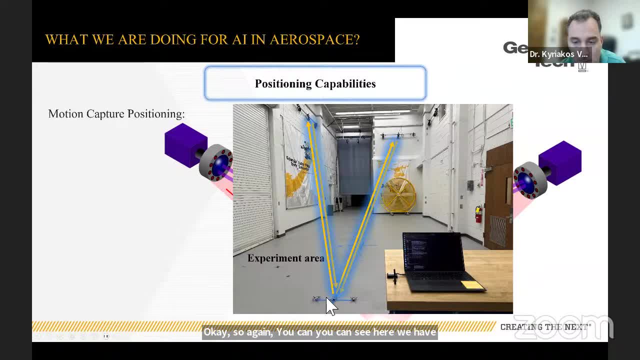 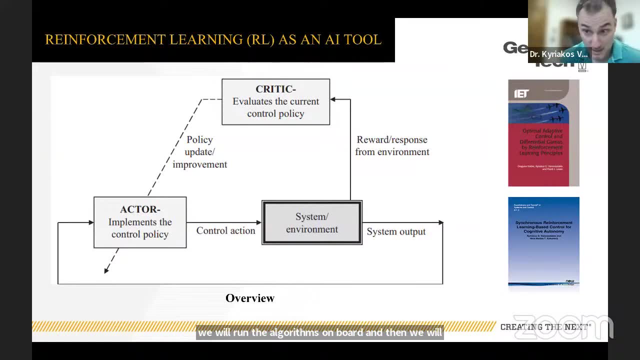 the cameras will locate them and then we will run the algorithms on the board and then we will see if we're successful or not. Okay, so reinforcement learning has been an AI tool for years. So, reinforcement learning- I'm sure you have all heard about Pavlov's dogs. 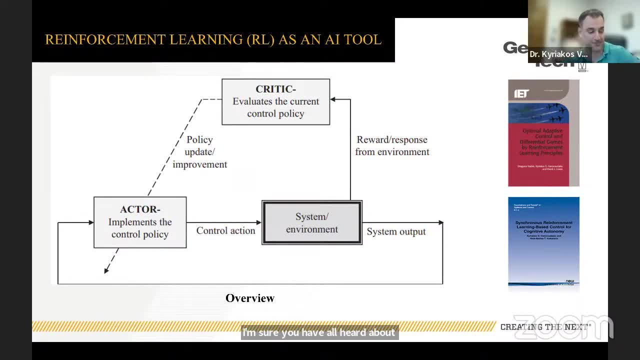 where he was using reinforcement learning to train his dogs. right, And so this is what actually every human learns, right? You use body words. So let's say that if you walk around and you hit yourself in the corner of the table, then next time you will not do it again, right? 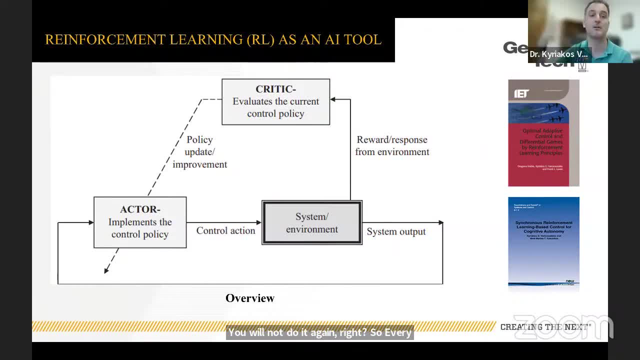 So every time you're improving and every time okay. So this is what we want to bring into aerospace: We want to make this cognition that it makes the system smarter and smarter. okay, So remember that here, instead of having this system environment. 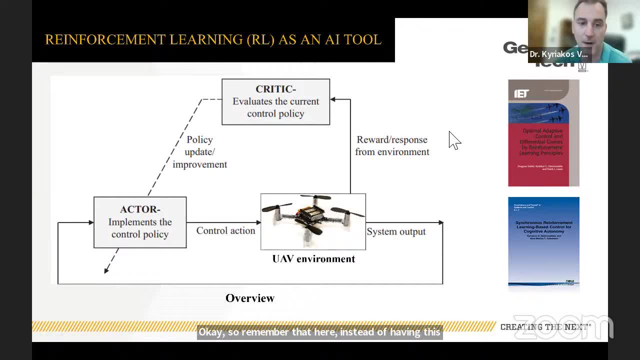 we can have any system that you can think And then for us we can touch it with our little baby drones. So again, we want to make everything autonomous, okay? So we don't want to have any offline computations and we don't want to be 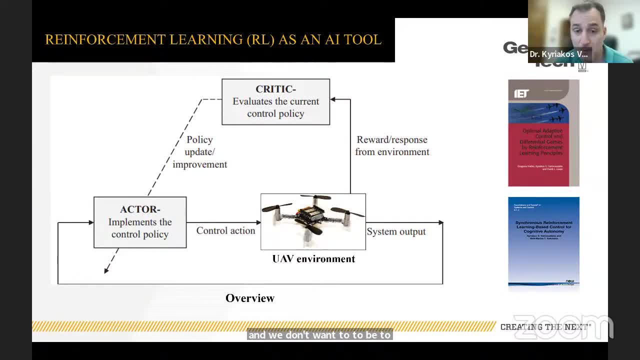 to have, for example, problems with robustness and stability. So what we want to do here is we want to have the RL agent, the reinforcement learning agent, to pick an appropriate control action. okay, So in reinforcement learning terminology this is called an actor, okay. 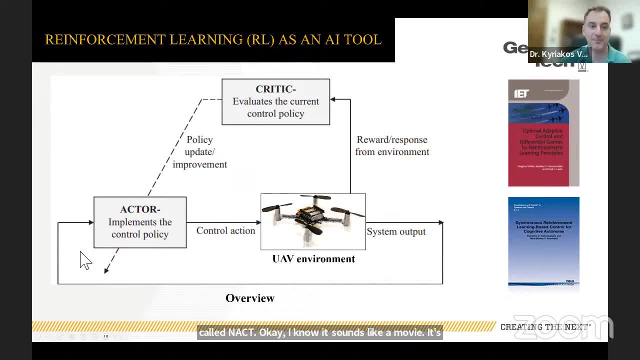 I know it sounds like a movie, but it's not okay. And then how good you're doing will be actually evaluated by something that we will call as the critic okay. So you can think that these two are smart structures, okay. 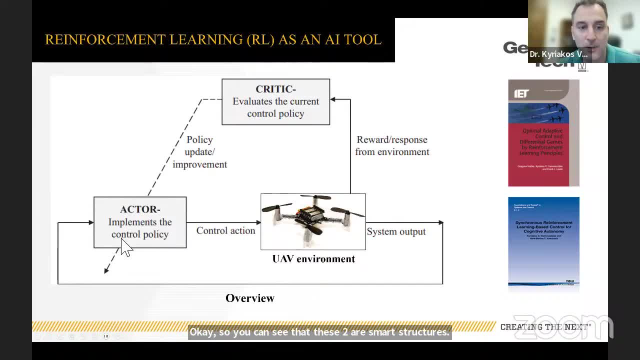 And they will tell you: okay, so the controller that you put into the system is not as good, so improve it, okay Again. and this works in a reinforcement learning way And you can see that the feedback that I talked before- right. 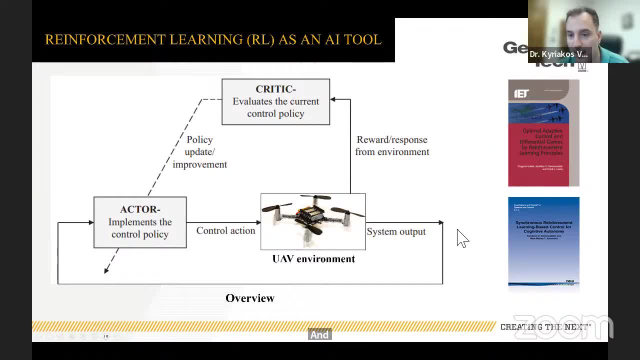 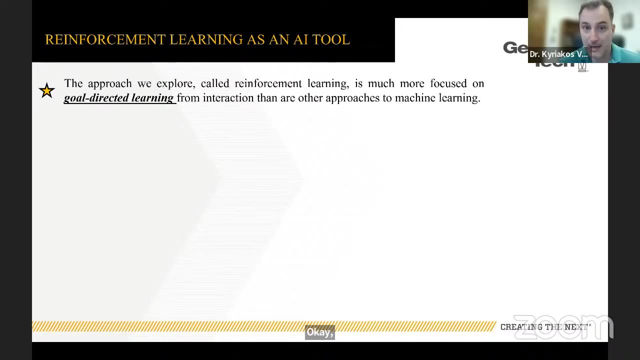 So, again, I have my sensors here. They send information back to my controller and, based on what my sensor said, I will improve my controller. okay, Okay. so, as I said, okay again, this is a goal-directed learning, okay. 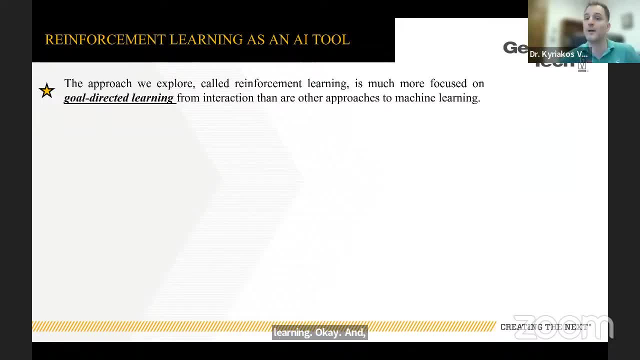 And it's actually the only, from what I can see- is the. I believe that's the only one that can achieve full autonomy. okay, So supervised and unsupervised learning. they require lots of pre-training and they cannot achieve a robust and stable autonomy. 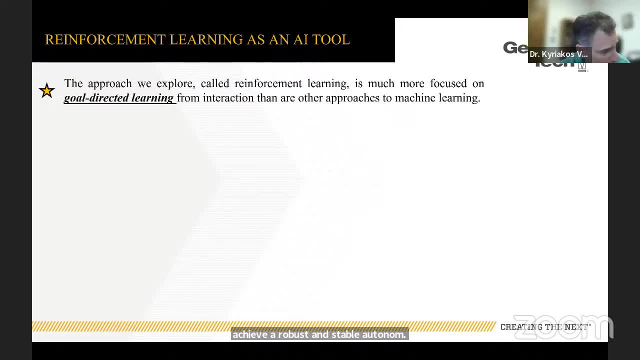 Also, I'm sure you have seen the accidents with the Tesla, where I think probably that was like five, six years ago, where they crashed on a track Because that was not trained properly. okay, So again what we want to do. 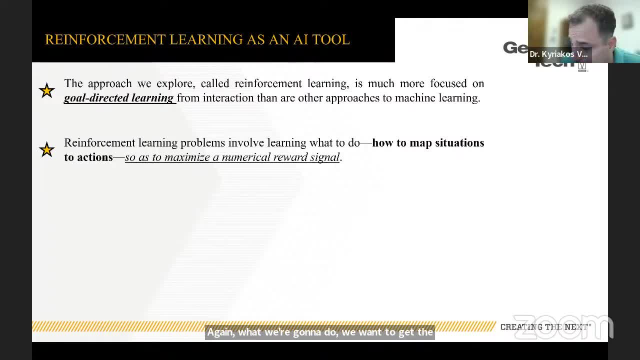 we want to get the best reward right. So what I mean by best reward is sometimes the best reward is to get the least fuel possible right, Or go from point A to point B in the minimum time, or different things. okay, So again what we want to do. 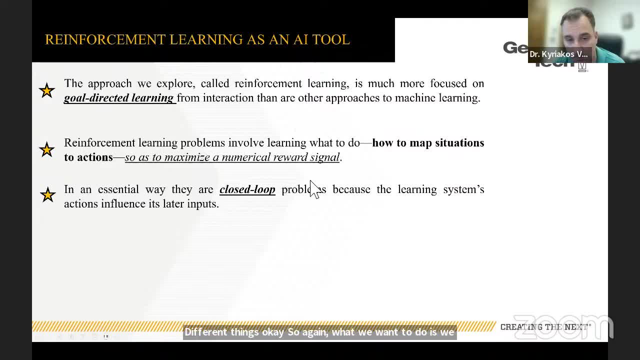 is: we want to have this feedback loop. okay, This feedback loop will let us influence our actions based on what our sensors are doing. Again, by influencing actions, we mean changing the actuators. Okay, so again, we are not told what actions to take. okay, 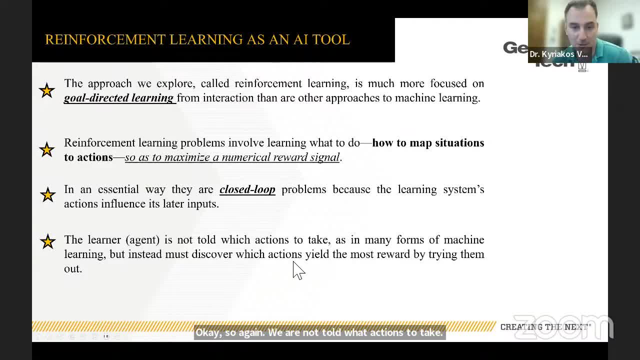 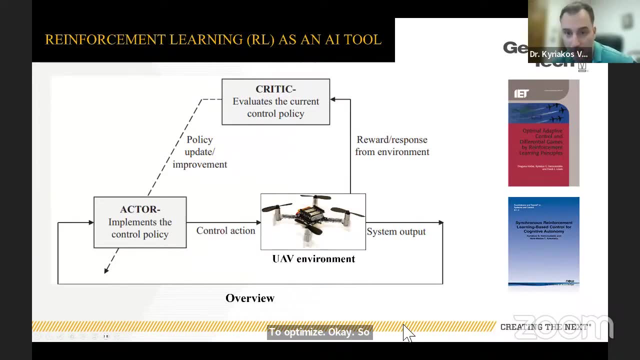 We don't say to the controller or agent what actions to take, but it will discover which actions to take based on what we want to optimize. okay, So again, remember that we had a reward right: The reward: we get a response from that environment. 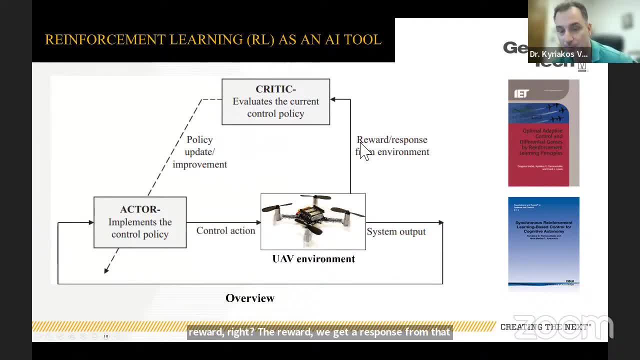 And based on that I make my next decision. okay, I don't say what exactly you have to do here, I just tell you: okay, you have a reward. okay, You pass it through something that we'll call accredit. 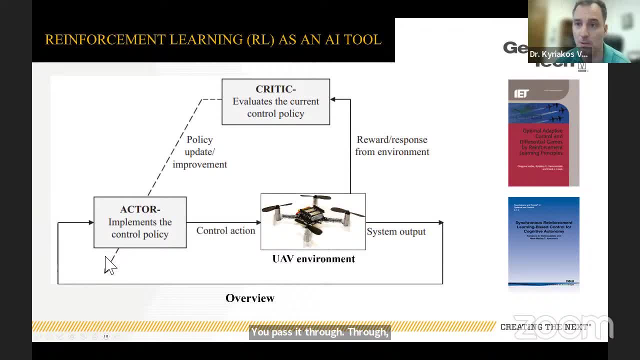 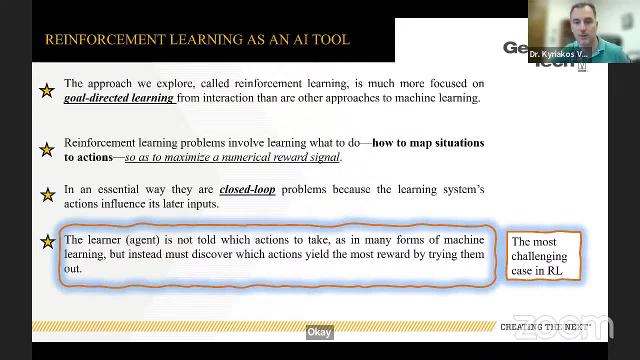 And based on that, I change it, And based on that, I change my control. okay, Okay and again. this is the most challenge from everything, right, So to discover by itself what is the best action to do. So let's see something. 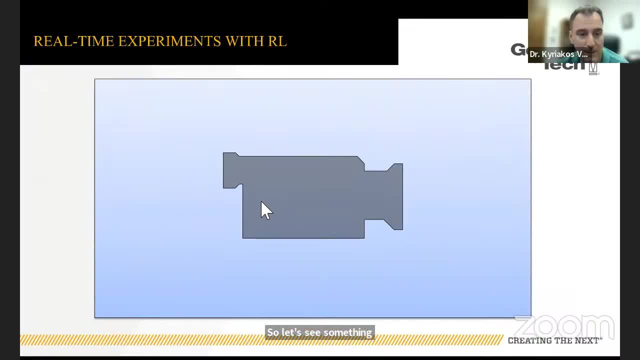 that we actually did a small experiment. Hopefully you can see my screen right now with the little drone flying around. I see your screen. I do not see anything moving around inside your screen, Okay, okay, So let's see why. So you see a video or you see just the PowerPoint? 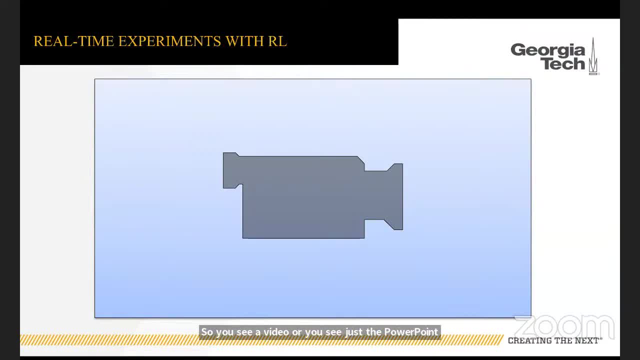 I see the what looks like a silhouette of a video camera in my mind: Okay, okay, Against the blue field, I don't see anything inside of it. Okay, okay, okay, Okay, that's, Let's see. how can I do that properly. let me see. 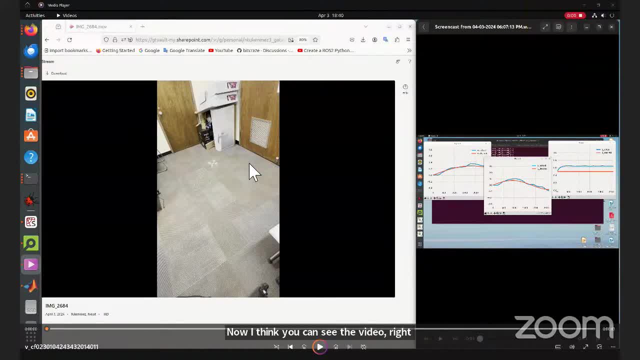 Now I think you can see the video, right. Yes, now I see the video. Perfect, okay, So what I want you to see here is okay, so we have this baby drone that you see it here And here on the right. okay, so I want my drone. 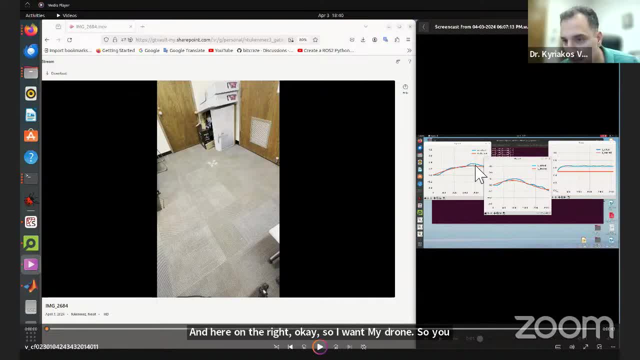 So you have X, Y and Z directions right. So the red line is the desired lines, okay, And the blue line are the lines that the learning will achieve. Okay, of course these are noisy aircrafts, okay, So of course, nothing is ideal. 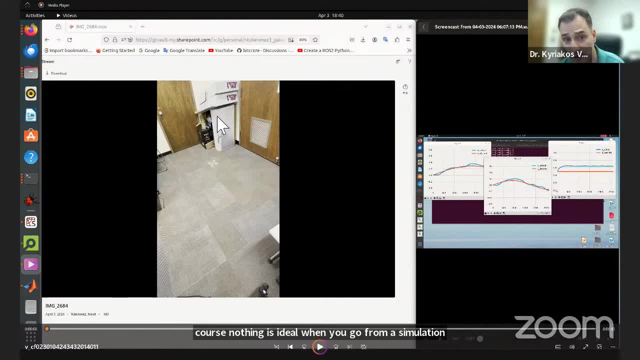 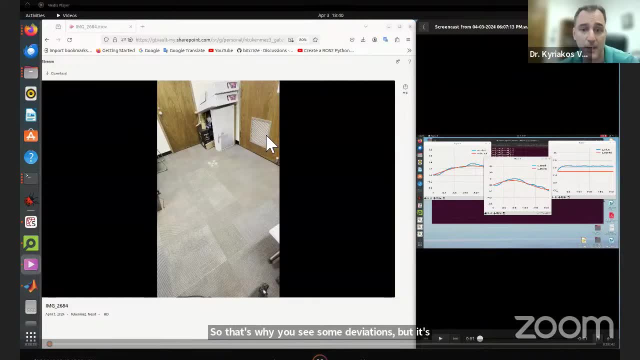 when you go from a simulation environment to a real hardware experiment. So that's why you see some deviations, but it's eventually learning, So let's actually run it. So here you see it flying. So here you see it flying. 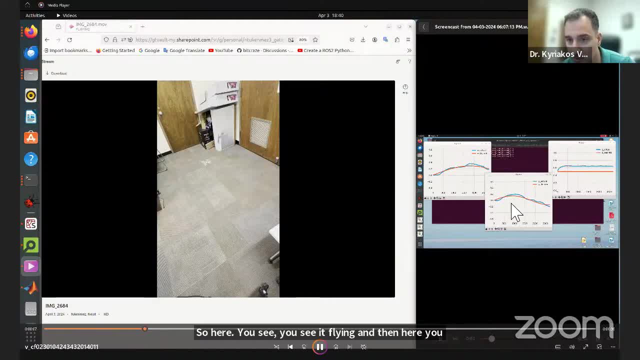 And then here you see how good the tracking is okay. So again, this is the X, this is the X direction, this is the Y direction and this is the Z direction. okay, So you can see that it tries to learn. 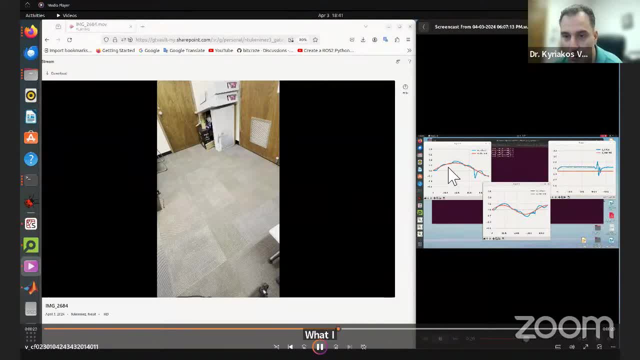 what I want it to learn. So again, I want the blue to be very, very close to the red line, okay, And again we're talking about X, Y and Z. So I mean here I want it to do just: 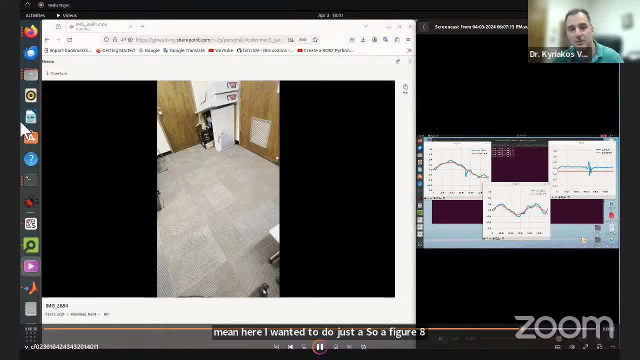 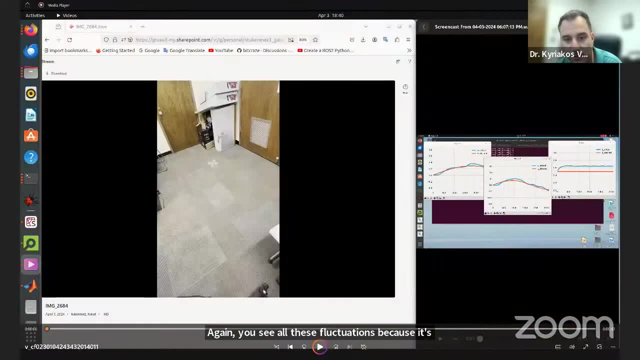 an eight shape, so a figure eight, and eventually it will do it Again. you see all these fluctuations because it's learning real time, okay, So let me do it again. So again you see the red lines, which is the desired one. 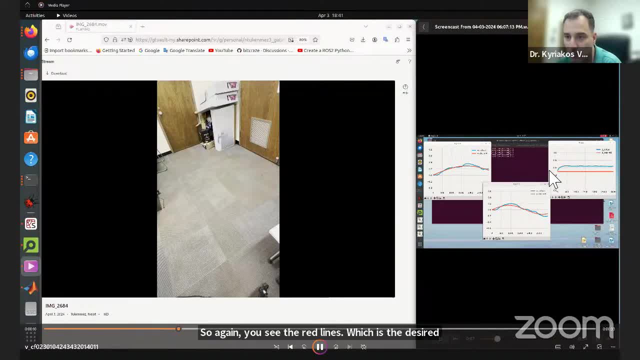 And then you see the blue lines is the actual, the one that it will do with the learning. Again, I haven't put any offline computations. Everything happens in real time. So the drone learns in real time how to perform a set eight figure. 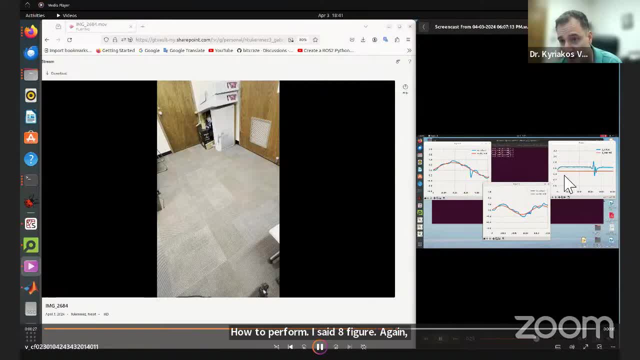 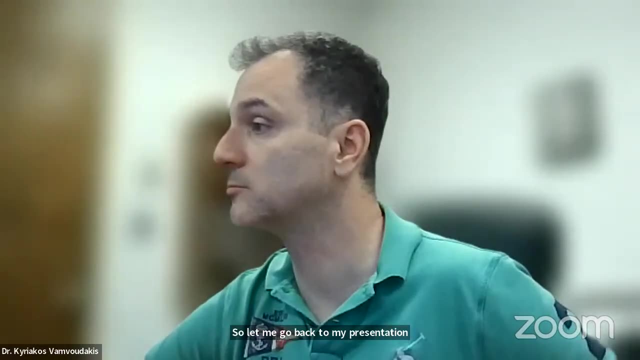 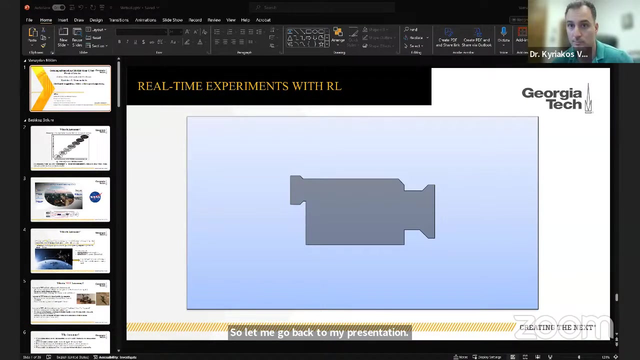 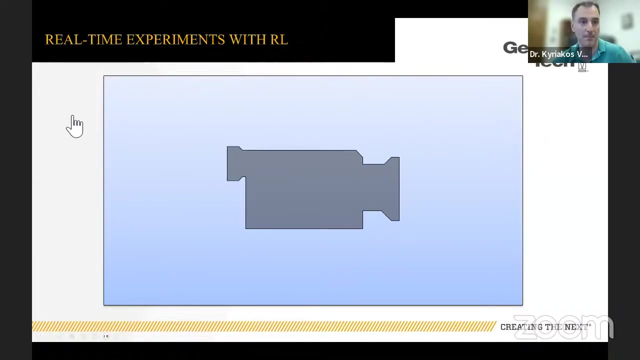 Again, it tracks the X direction, it tracks the Y direction, it tracks the Z direction. So let me go back to my presentation. I think now you can see my presentation back. right, That's correct, yes, Perfect, perfect. 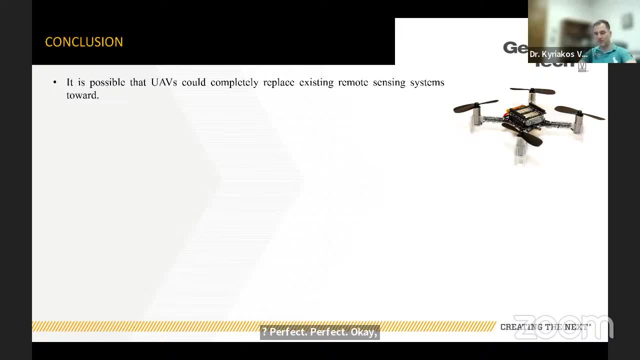 Okay. so again, what I want you to show is I want to give you a background of what's autonomy in aerospace, what we consider autonomy in aerospace, because different people consider it different, okay, So I want you to emphasize okay. 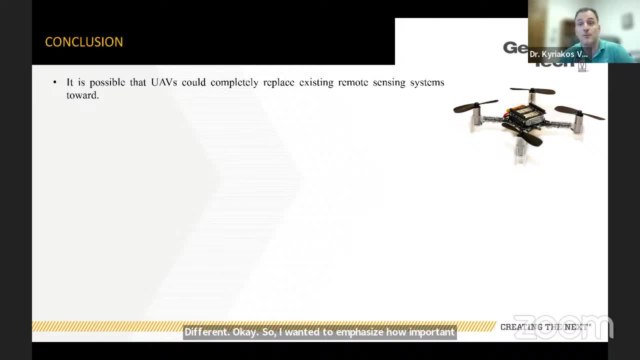 how important security is in aerospace, And I want to show you also how we can manipulate even these little small drones to do what we want with reinforcement learning, okay. So again to conclude, so I want to emphasize that UAVs can potentially completely replace existing remote sensing systems. okay. 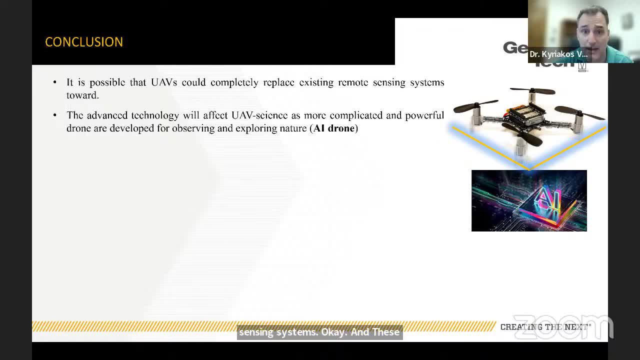 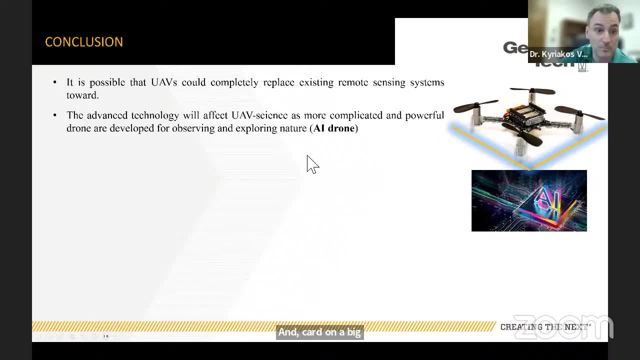 on a bigger drone what I could do- okay. And of course, we will resolve lots of things that right now they're not solved during autonomous flights, for example, obstacle avoidance- okay, How to do long term missions and how to make smart decisions in a formation. 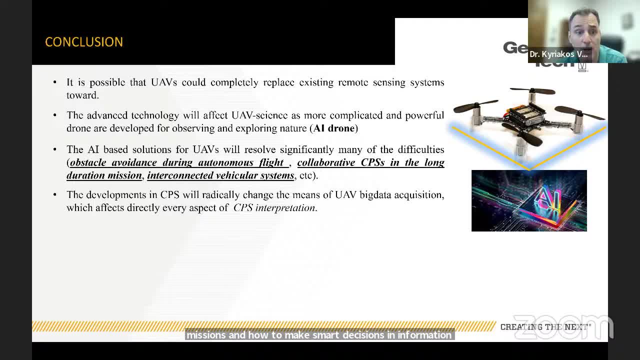 and so on and so forth. So what I think also is that if we consider the interaction of the physical and cyber parts in a different way, then we can potentially change these UAVs, the swarm of UAVs and, in general, aerospace okay. 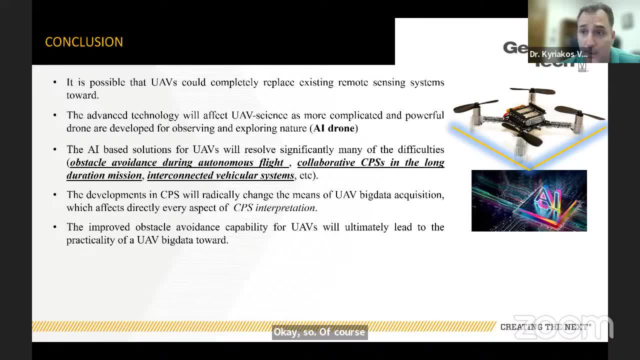 So, of course, every time, you know, every time, you know, every time, in an urban air mobility scenario, you have all these obstacles, these buildings and so on and so forth. Every time you go around all these buildings, you can exactly, ultimately lead to the practicality. 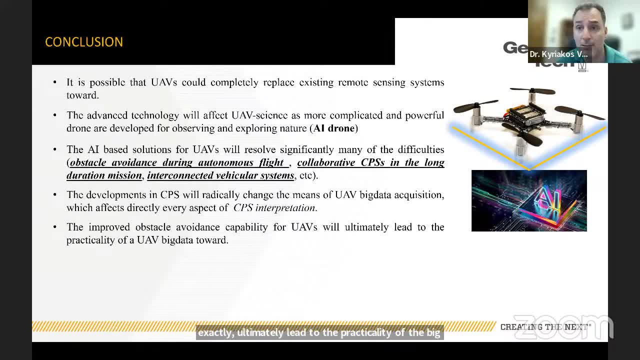 of the big data. okay, So all these things, they will give you lots of information of how, what happens in situations where you have a conflict, obstacles, and so on and so forth. okay, So again, every day there are more things coming up in the UAV scenarios. 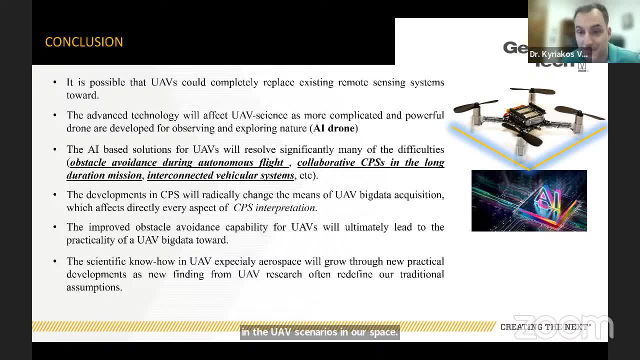 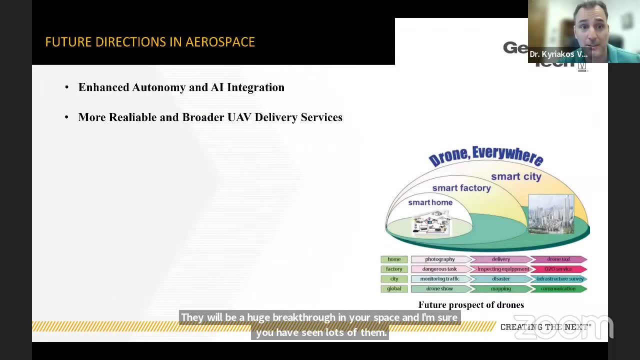 in aerospace. so as we get more intuition and insight of what is happening, I think there will be a huge breakthroughs in aerospace, and I'm sure you have seen lots of them, and then we have lots of things that we're planning to work on in aerospace. 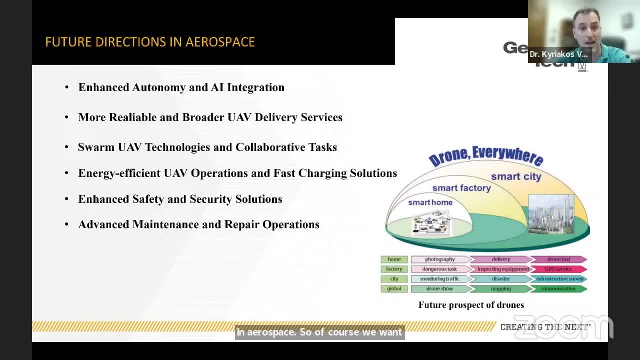 so of course, we want to enhance autonomy and how AI is integrated with the cloud. We want to make sure we are part of that necklace of Faculty Citizens and Labor Code, and then we want to make sure we are part of that necklace- autonomy. We also want to work on UAV delivery services and how to make it more reliable. I'm 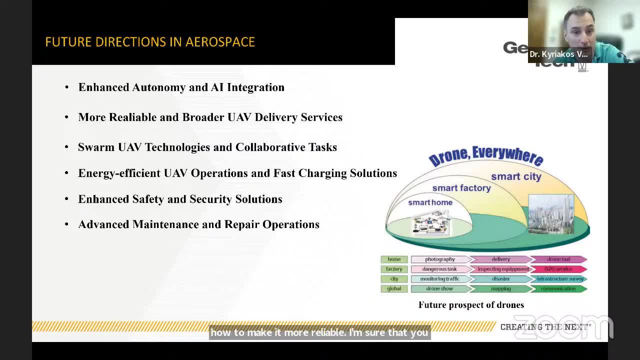 sure that you have seen lots of hype about that as well. We want also to be very efficient when we do these UAV operations, And if they're battery operated, I want also to make sure that we have fast charging capabilities. So one other project that we actually had was 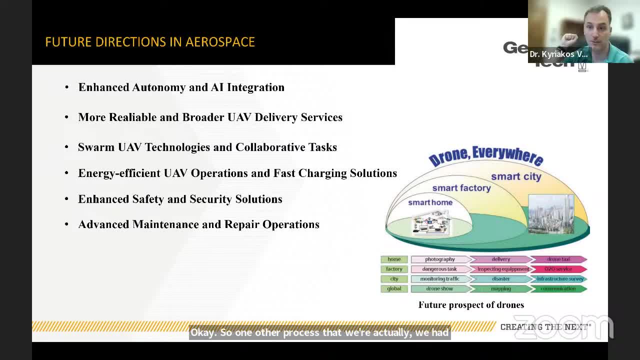 on securing fast charging stations from attacks. that can happen either for cars- fast charging stations for cars- or for drones- And of course, we want to have advanced maintenance and repair operations and general UAV solutions. And then I think I planned for a 45-minute talk. 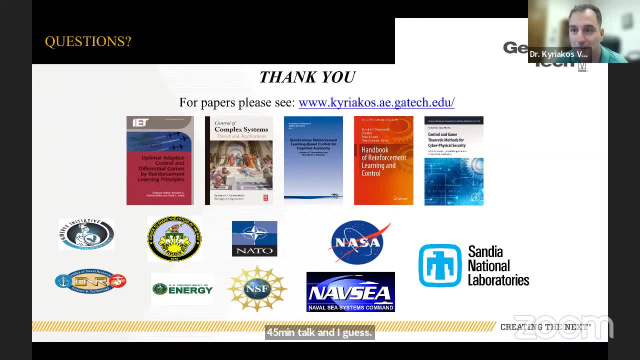 and I guess It was 50 minutes, but I will be happy to answer any questions. Oh, that was fantastic. Thank you, Kriakos. We did get several questions in, so I'm going to take them in the order that they came in. 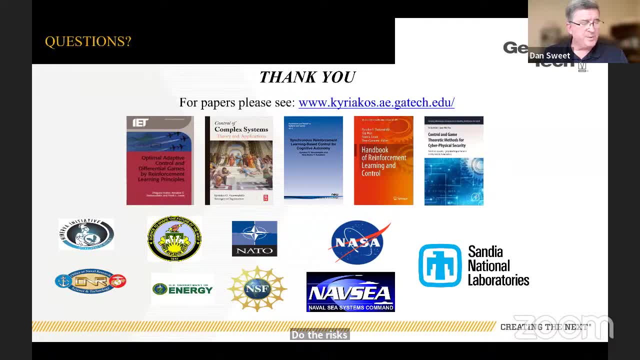 Do the risks of vehicle-to-vehicle communications as a new threat vector outweigh the benefits providing situations? Okay, So to understand the question, so every drone or every UAV, it has different communication capabilities and how this can affect security of the whole team. Was it that? 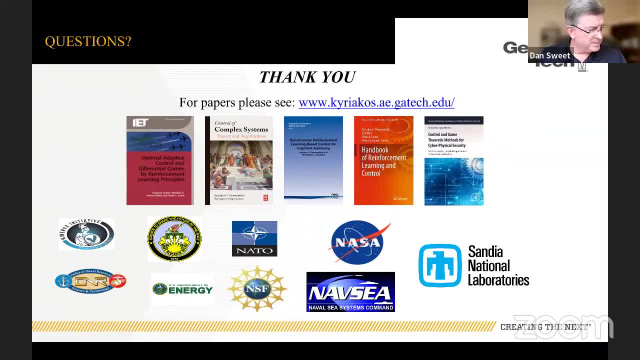 question. The question again was: do the risks of vehicle-to-vehicle communications- Okay, as a new threat vector- outweigh the benefits? providing situational awareness, Okay, Hmm, Again, the S2A2 project is about doing these flying cars, So 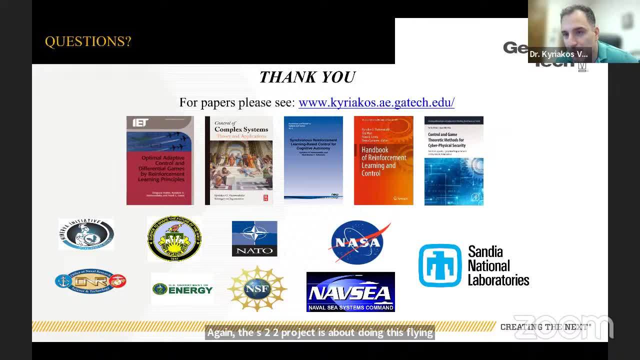 maybe they can actually explain the questions more. I don't know what exactly. Okay, The person who asked that question. if he doesn't mind providing a little bit more information in the chat, we will go on to the next one. Sure, 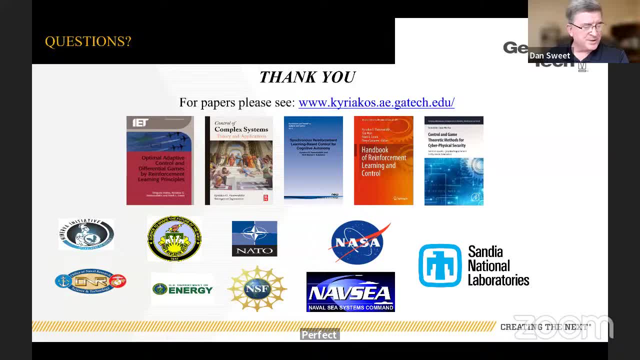 Do you see the use of emerging open ATM standards, such as ICAO's SWIM, as increasing cyber risk in our airspace or reducing it, and why? Oh, I mean, I think it will increase Every time we have something like that. it will always get. 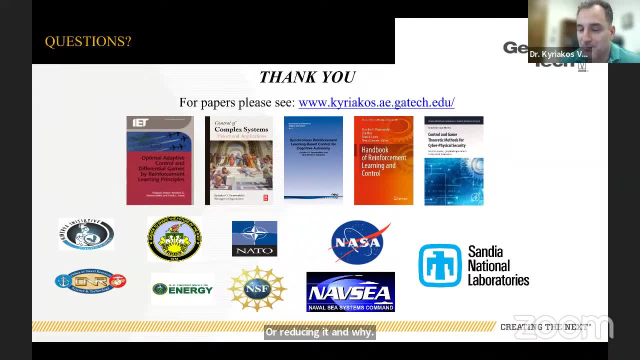 attackers smarter and they will always find ways to get anything, So I think this will potentially get more doors for threats. Okay, The person did respond back on question one and basically he's saying: have the risks of vehicle-to-vehicle communications been examined? 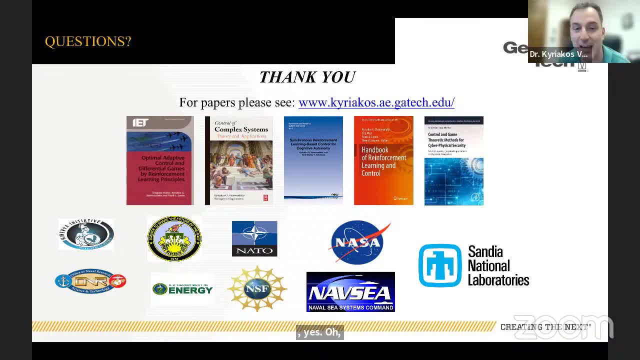 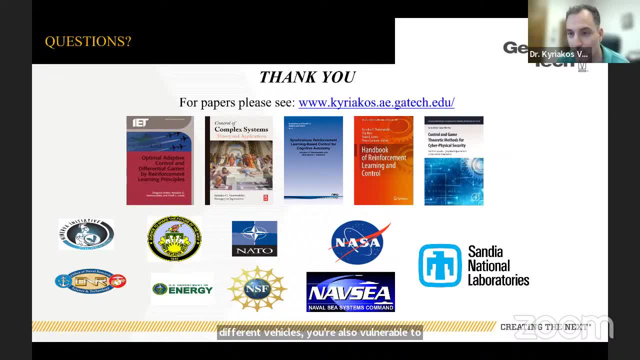 And you're vulnerable to several, for example, denial-of-service attacks and so on so forth, because if I want to send information of position and velocity from one drone to another drone or from one flying car to another flying car, okay, so this can also be jammed by adversaries. 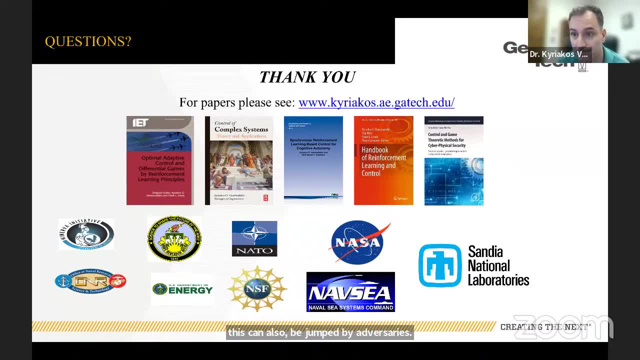 So, yes, we consider also communication attacks. This is a question of mine. It seems like right now there's, particularly in the Middle East and Europe, there's a great deal of gps spoofing going on. is that, um, how did i phrase it? is that an example of a threat to a cyber? 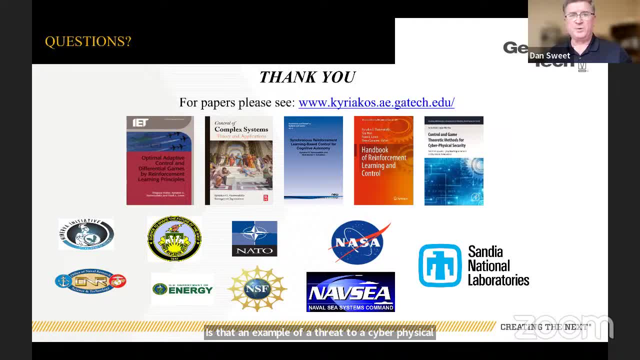 physical system. is that a product of ai programming or do we know how that's being accomplished right now? okay, so that's a very good question. so, um, we have a lot of work on gps, uh, gps spoofing. actually before i was at virginia tech and we examined how you can spoof underwater vehicles as well as 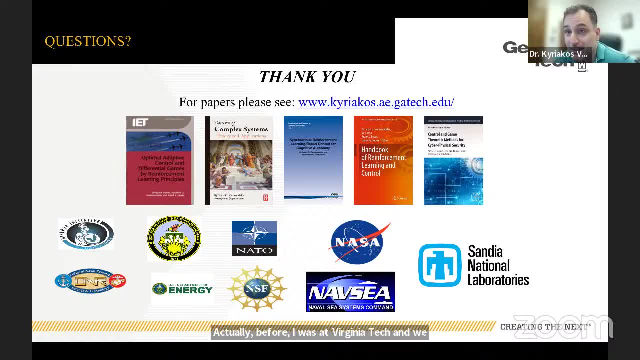 drones and spoofing can be actually mitigated. if you have multiple gps receivers on on board, okay, and then what you do is you put them on different locations and then, based on that, you take a visiting agreement between all those. so, because the attacker has to actually either spoof, 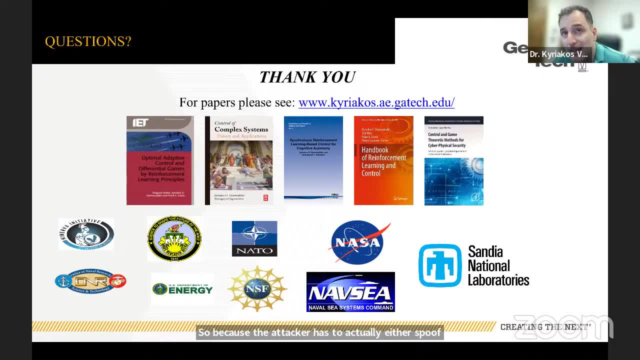 all of them together. but he- he mostly- doesn't have the capability and the bandwidth to spoof all of them together. so he has to spoof all of them together. and then he has to spoof all of them, okay so, all of all of their targets that have limited bandwidth. okay so, because they don't. 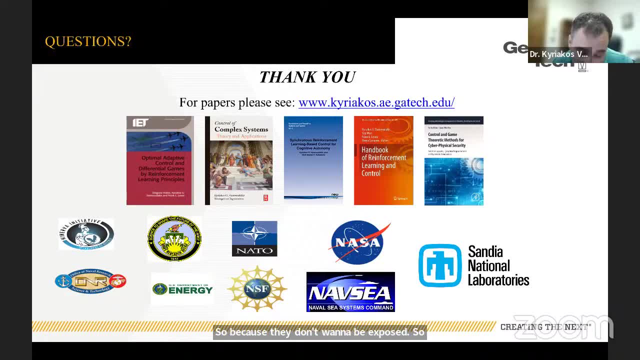 want to be exposed. so, um the time that he, he or she spoofs the gps, then you will be able to see, by visiting agreement, you will be able to see from the other gps that something wrong is happening. okay, so actually, the aircrafts. they actually use multiple components right now. 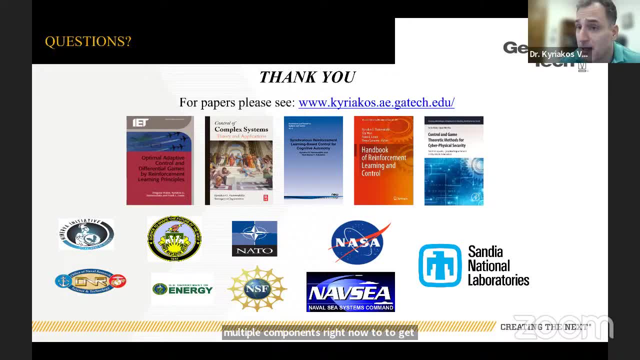 um to to get a visiting agreement between all these things in case something goes bad. but i remember at at virginia they had a colleague who actually spoofed um a very large super yacht. so what they did is: um uh, they have been working on gps spoofing for a long time and then they found a very rich person and then he's like: if you can, 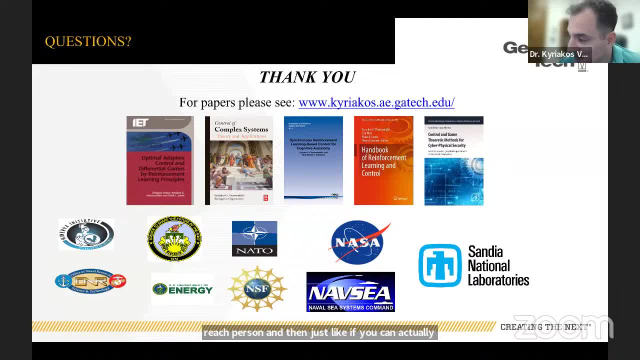 actually spoof my super yacht. i will let you have two weeks free vacations, so- and then they were cruising in mediterranean, and then they will use news all over that. so if you google super yacht spoofing, you will find it, and so what happened was that he was, they were. 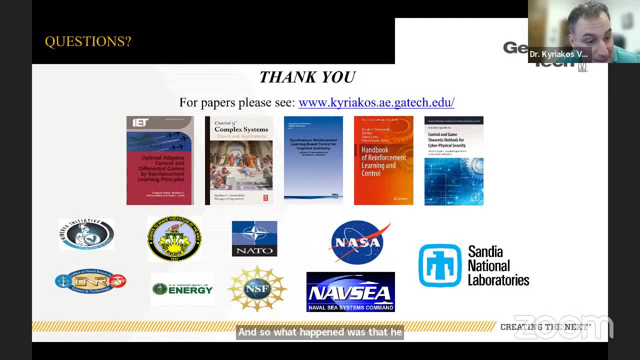 able to spoof it and uh, the the captain thought he was somewhere else, but they were actually deviating from this area and um, so yeah, and it was all over the news, uh, so if you're interested on this one, that will be fun to watch i might have to take a look at. uh. 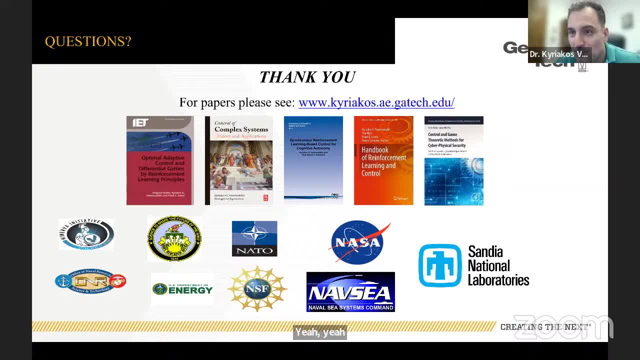 take a look at that, yeah, yeah, we have another question for real-time airspace networks. do sims tell us resilience to weather events is better handled by centralized ground ai control or by decentralized, distributed vehicle ai control? okay, yeah, that's, that's a very good question as well. so again, the more decentralized and distributed you are, 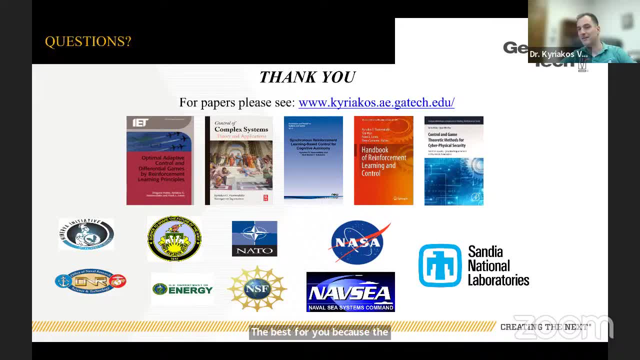 the best for you, because the attacker or whatever adversary you will have, will have to change all these things. okay, if you have only one computer, a centralized information, the time that the attacker spoofs, changes or does something in centralized information, then your whole mission would probably be in jeopardy. so, having more distributed information, 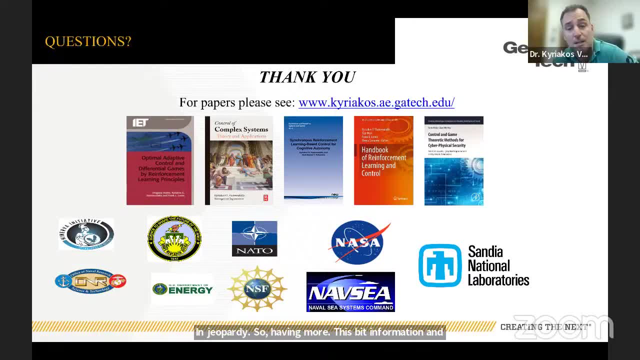 and having visiting agreements. between all these things is is one key to mitigation of these attacks. we also had, uh, a person ask a clarifying question. can you explain the difference between automation and ai again, please? yes, yes, yes, yes, yes. so automation, you can think that when you are at your place and you actually change your temperature to 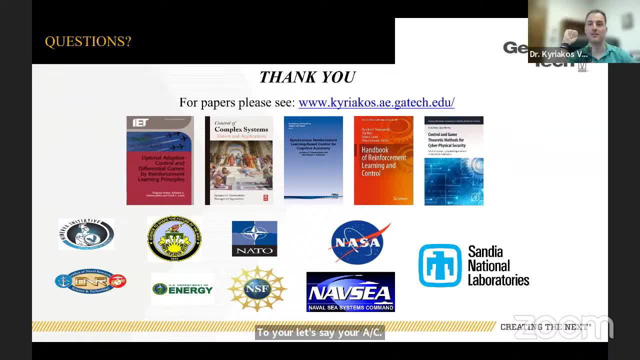 your, let's say, your ac to 69 or 70 degrees, right, so you will eventually reach this temperature, right? um, so, this is somehow like a small automation, okay, but there is nothing smart in this one. so the time that you put something smart into automation- like, for example, i'm improving over time, okay, so, uh, i'm learning over time, i'm getting better. 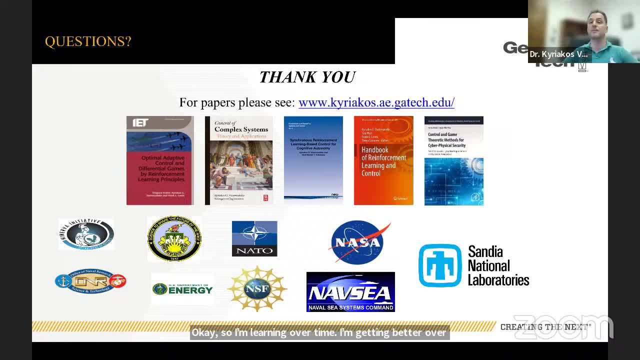 over time. so i will not do this mistake again. so then, and only then, you have a complete autonomous. so i will say that the time that incorporate cognition in all these things, it's, um, it's, it's the answer to uh, to autonomous systems. okay, let's, uh. we'll start wrapping up. i got one more quick question just to my own. 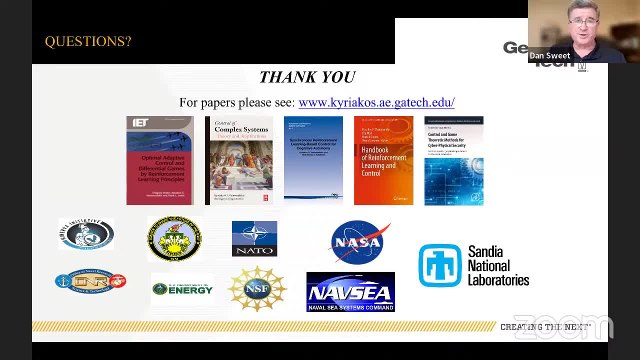 uh, and maybe this is a maybe something for either a personal response or something on behalf of nasa. where do you think the majority of threats to aerospace are going to come from? is it going to be a corporate espionage issue, a government issue, or is it going to be the random individuals or groups with an agenda that will pose the biggest threat to 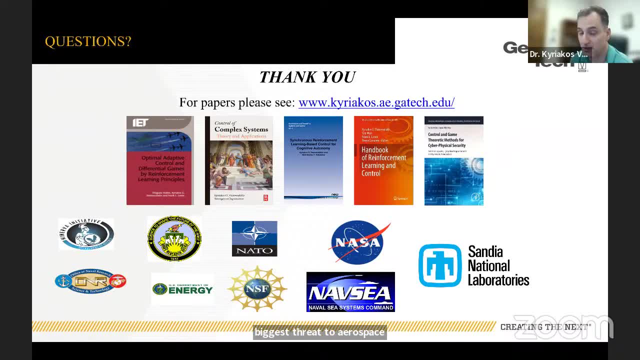 aerospace. i will say all of the above. i mean, and the biggest threat will be probably some teams with uh, with an agenda, so uh again, the most attacks that i have seen in several uh drones and so on, so forth. again, they have been from china and russia, but uh, i don't know if it was. 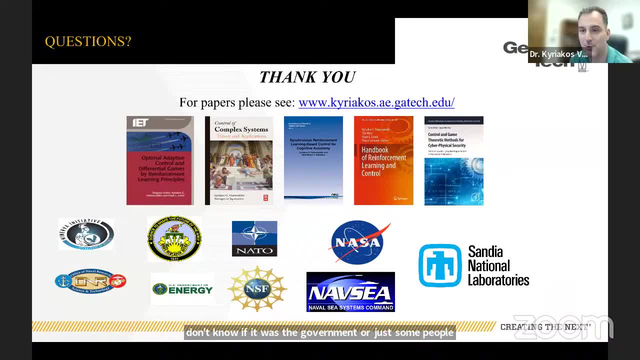 the government or just some people. they're just some teams, they're trying to to get information about things. so uh, but yeah, so it's, it will get worse. so uh, but yeah, i mean china, russia, they're the responsible ones. but again, we cannot link it back to to the governments, but we can link 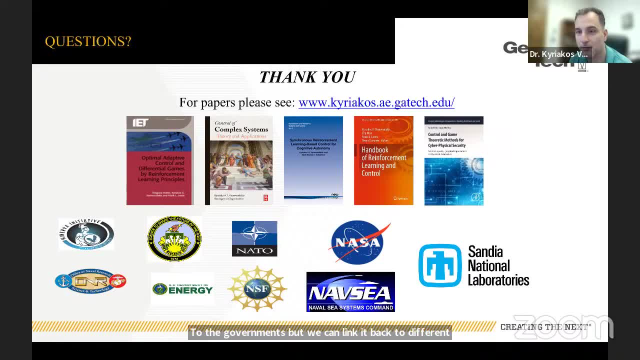 it back to different groups that they try to get information of several things. okay. well, uh, i can't tell you how much i appreciated this today. dr van vodakis, this has um been a really interesting topic. a lot of it uh went past me, i will freely admit uh. but no, i really enjoyed uh. 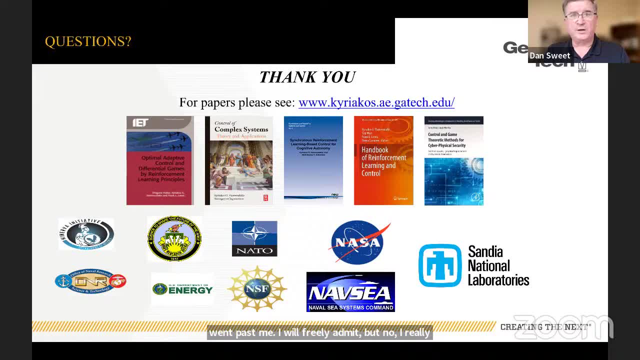 hearing it on the topic, knowing where our aerospace industry is headed now. obviously, things have changed significantly in aerospace over the years and, uh, it's going to continue to change and we have to adapt and overcome to keep flying. so, uh, appreciate your time today, appreciate the work that you and your team are doing in the. uh, the work that your 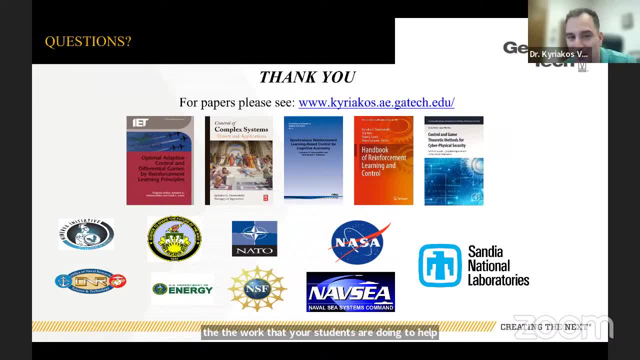 students are doing to help for the future as well. thank you very much, dan. thank you everybody for being here again. i'm- uh, i'm always available. if you guys have any questions about anything, i think you can find my email or my information online and then you can send me an email and i 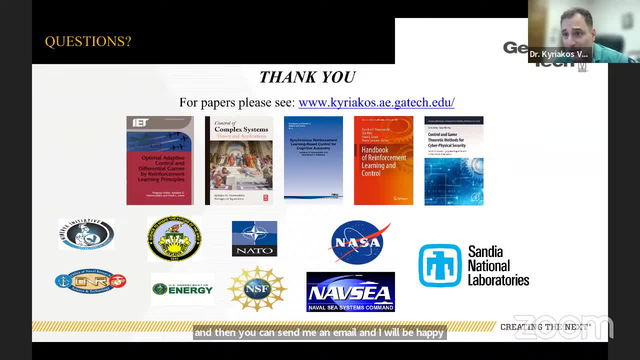 will be happy to uh to uh, to talk with you or answer any questions that you might have. one real late question came, sure, on charging security. you examined the s the 2022 sandia report on ccs, and do you believe iso 15118-2 would fix it? 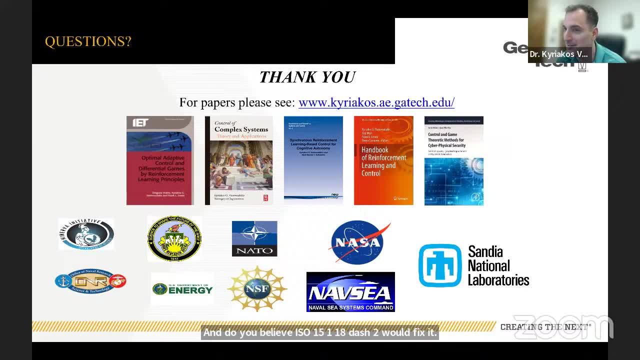 uh, to be honest, i'm not familiar with that, but i can check. okay, i might get that person's uh email address to you. uh, sure, yeah, i mean it sounds like you. you provided the information on how they can contact you. yeah, yeah, yeah, yeah, okay, well, uh, again the. 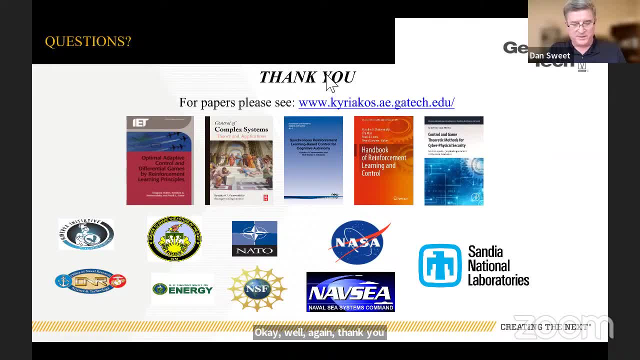 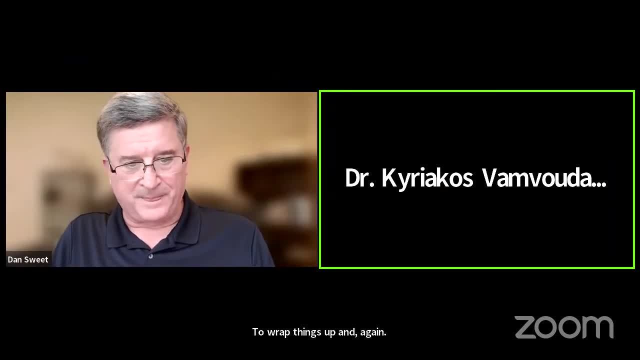 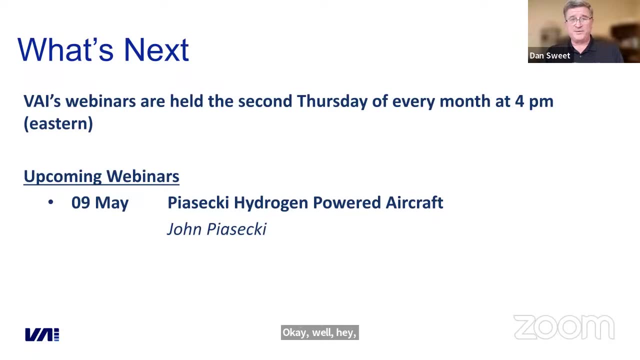 thank you for your time. if you want to stop sharing, then i will go ahead and start sharing my screen to wrap things up. and uh, thank you very much. thank you for your time. thank you, okay. well, hey, coming up next. uh, that number one. that was fascinating. 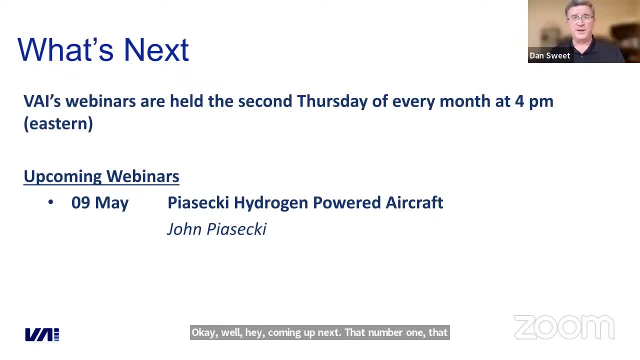 number two. we're going to stay on a technological theme, uh, with our next webinar. our webinars are held the second thursday of every month at 4 pm. here we are today. uh, the next webinar is going to be on the piasaki. how hydrogen-powered aircraft? uh, right now it's under development: the pa 890. 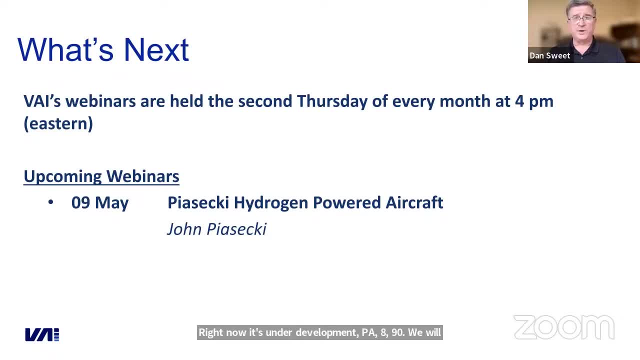 we will have uh john piasecki from the company joining us to talk about that development and, in the future, of hydrogen-powered aircraft in general. um, we i know that he's working with zero avia on their hydrogen fuel cells, and so there's the potential for a great deal. 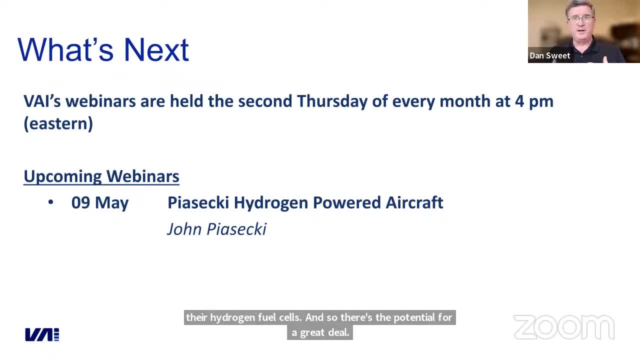 to me, hydrogen-powered aircraft are going to be coming in faster sometime in some cases than maybe battery powered, but i believe they'll also have different applications and so, uh, getting to learn a little bit more about the hydrogen-powered aircraft should give us an insight on where. 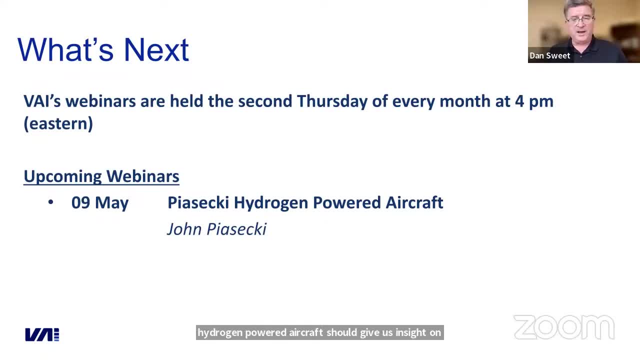 the industry is headed. look forward to that one as well, and we're looking at topics such as um, employee retention and engagement for future ones. that would be something managers and workforce development people might be interested in hearing about, and we're also looking at a webinar coming up on for new pilots. hey you. 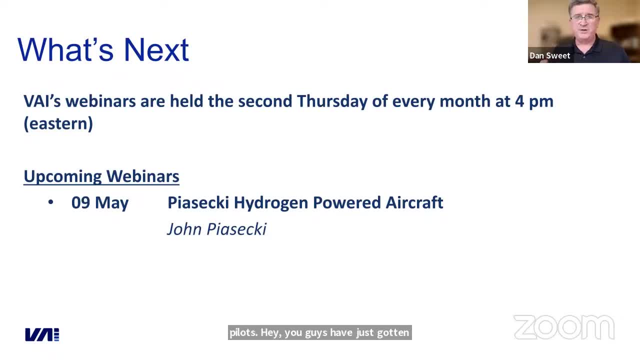 guys have just gotten your pilot certificate. you've got maybe 100, 200 hours. what's next? how soon before you can launch yourself into some of the bigger aircraft or more specific missions that you're interested in? so those are topics we're looking at. hit the button here, um. 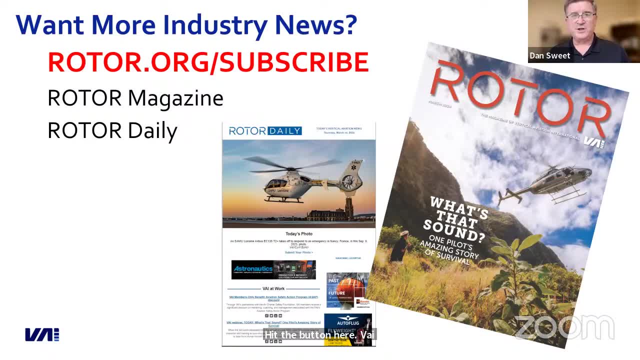 vai, we like to share information. we have a couple publications right now. one is print rotor magazine. we're going to be changing the name of it fairly soon, once we come up with the the right one. um, it's a quarterly publication, an award-winning publication, a lot of in-depth information. 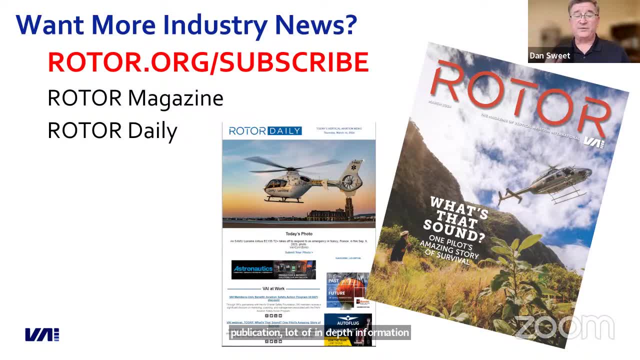 we encourage everybody to subscribe to that. it's free unless you live outside the united states. and then there is a small stipend uh included for shipping, international shipping, vertical. uh, excuse me, rotor, daily we, it's something we send out every business day. uh, we comb through uh the internet to find stories. 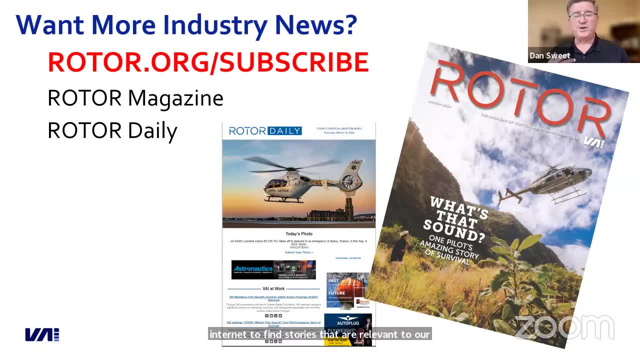 that are relevant to our industry and share those with you, so you don't have to do the searching uh. we've uh provide sources. you know google's obviously one of them. ai will probably be used uh more and more as well. um, we also reach out to the manufacturers. our hai.